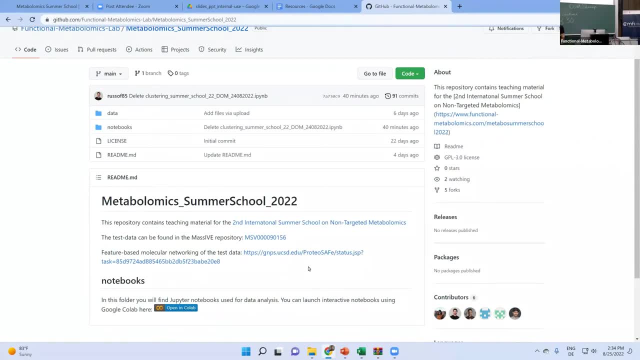 Are you alive, guys Surviving? Since there is a step for installing the packages, it takes some time, So we will just open the notebook and do this step first, so then we can come back to it. I will introduce the topic in the meantime, and then you have the. 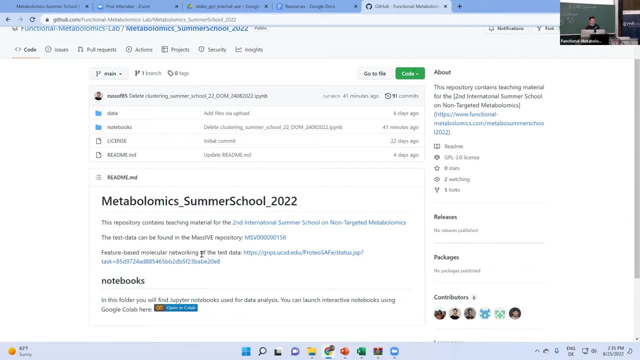 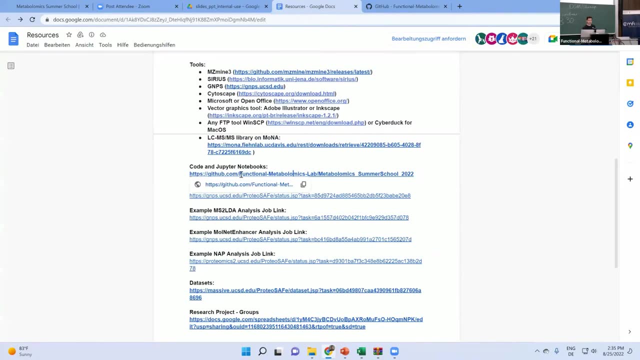 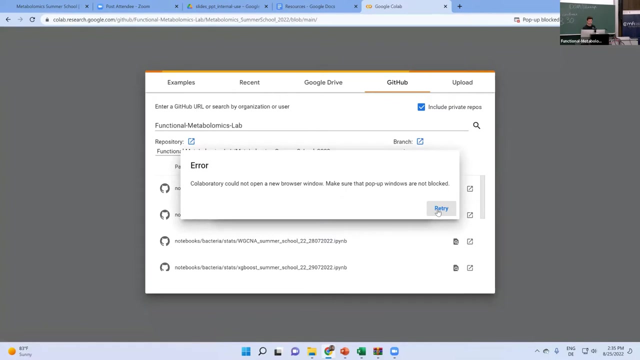 packages already installed. Okay, So are you in this page, in the GitHub page? Yes, You can go to the resources again and then the GitHub link And then you can open Google Colab And then there is only one file called clustering. so this time it cannot. 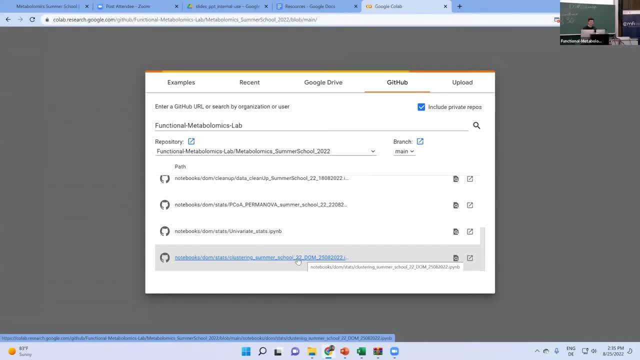 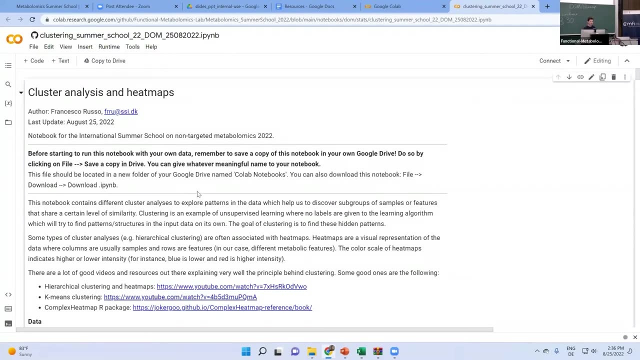 be wrong. Okay, No bacteria, nothing. Just click it here or here. it will open in another pop-up. You can see, I just updated a few seconds ago. It's important, as we said, that we create a copy And you can rename these as you want. 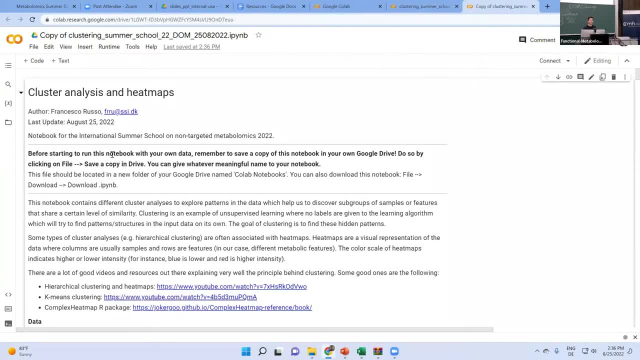 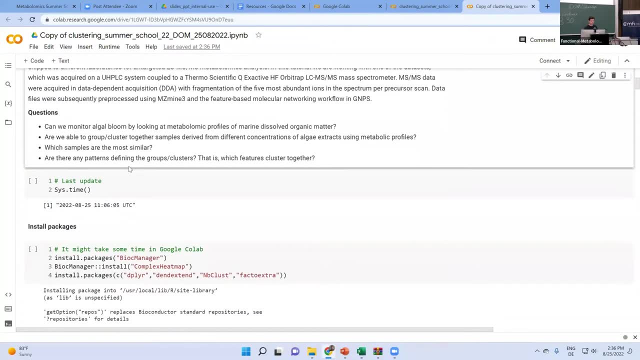 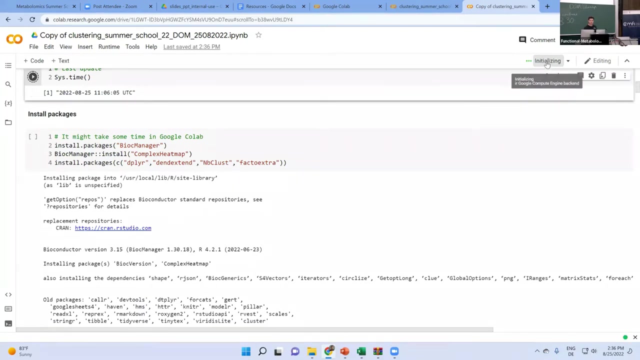 And it's really easy. you can just call it whatever you like. Oh, Are you all here? Yeah, So in the first step it's just To check for the time For the last update. As you can see here on the right, it's connecting to the runtime. So now it's ready And this: 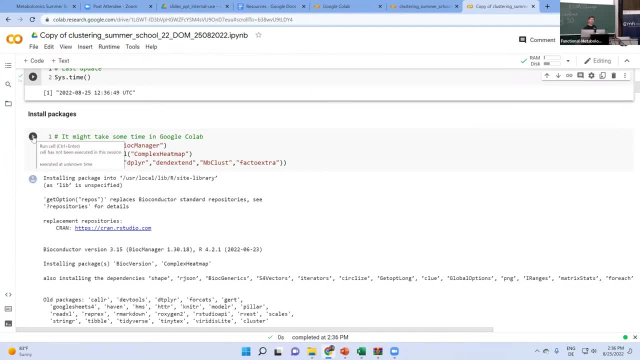 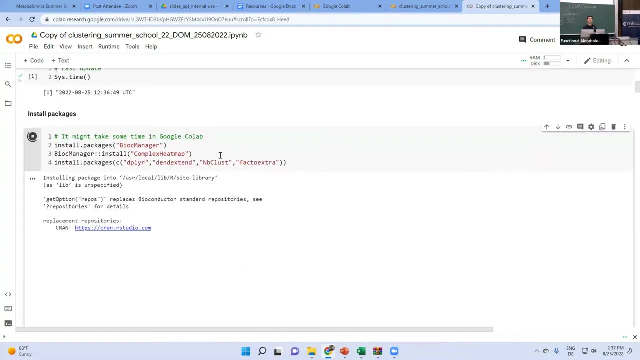 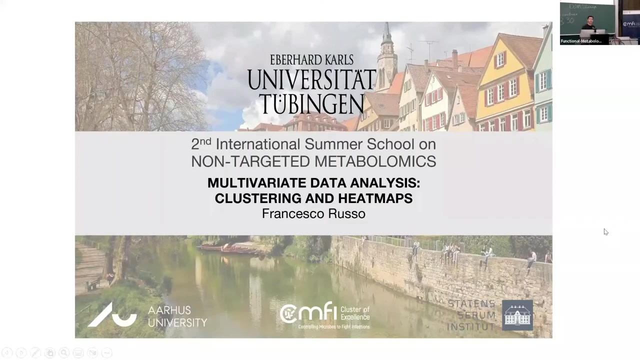 is the time connection. Okay, One second step. so just click on the packages and now we'll install the packages, okay, yeah, so I will introduce a topic now and then we come back to this. okay, so I would like to introduce some concept related to clustering and heatmaps, I know. 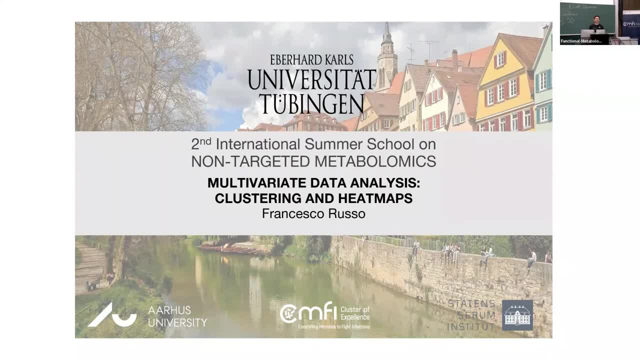 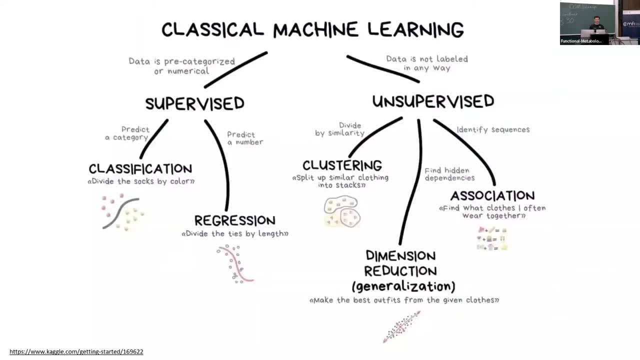 that for many of you would be trivial, for some others would be a new thing, and it's a audience, so we have to try to fit a lot of things inside and during this summer school probably, you heard a lot of terms. many of them can be under this umbrella of machine learning work. we 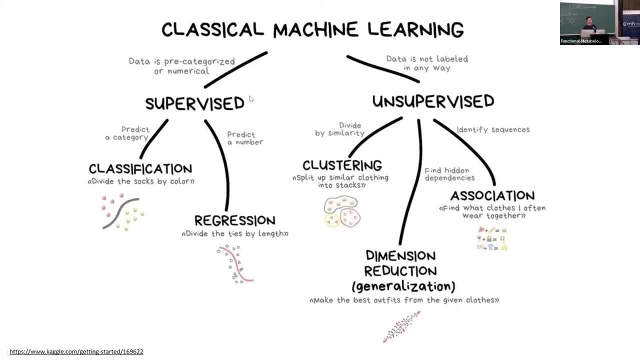 can say we can divide machine learning in two sides, so one supervised branch and one unsupervised branch, and the supervised branch basically uses a label to classify, in this case socks. if you want to classify socks by color, or you can also predict the number, like the length of the ties, for instance, and the part that 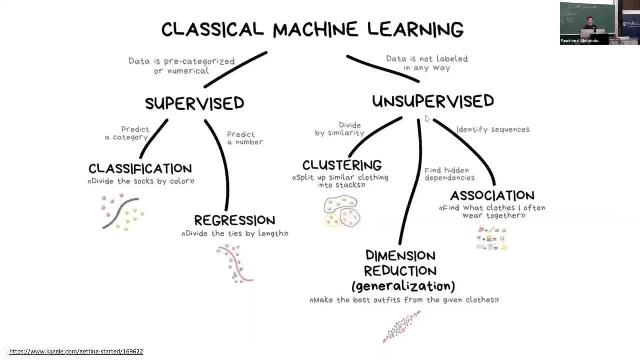 we are talking about today- actually Madeline already mentioned it a bit- is dimensionality reduction. PermaNova PicoAce is one of those, PCA is one of those and many others that you heard before Disney Yuma, and there are methods based on associations. so how frequent you. 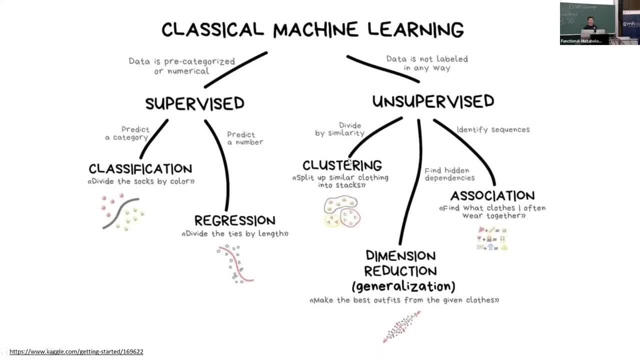 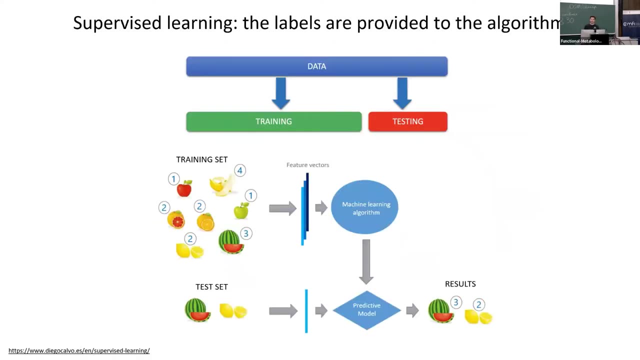 can find an object together with another one and you can also find the clustering type of objects you pay attention to within the learning branch here. that is the one that I'm talking about today. so we want to put, for instance, similar clothing together. the supervised learning, the labels are provided. as I said, you have your data and you divide. 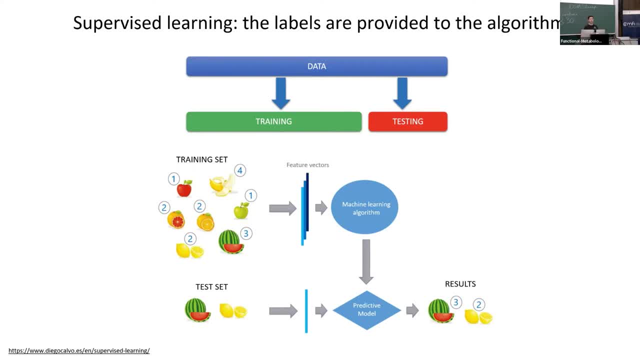 your data in training and testing. you build a model, mechanical learning model, based on the training. here we have a lot of type of fruits, and then we build whatever machine learning we want, and then we build a predicting model on the training and then we have a lot. of type of fruits, for example. machine learning, that is a protocol for tests and algorithms, in other words, which we lost, so hope you use it. well, we see some responses. we have to thank you guys. see if there are problems in other application and successful project님� North. but then we see yourself thinking together, wike. 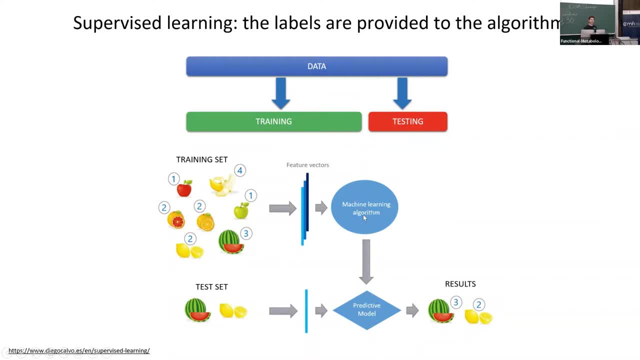 with Moritz yields, then is a match for Palestinians and similarly, folos protecting advocates, other companies depending on specific this. The test set is never seen by the model and is used to evaluate the performance of your model. This is a very generalization. of course, there are many more complicated ways of doing this. 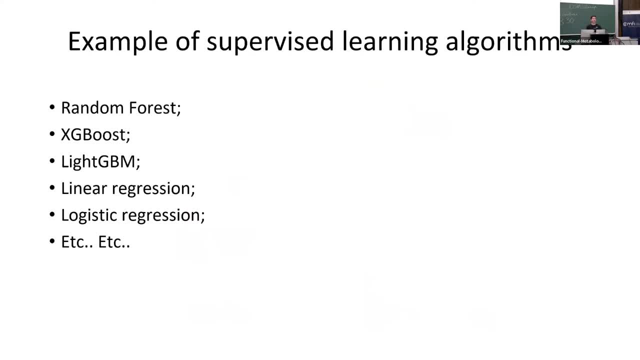 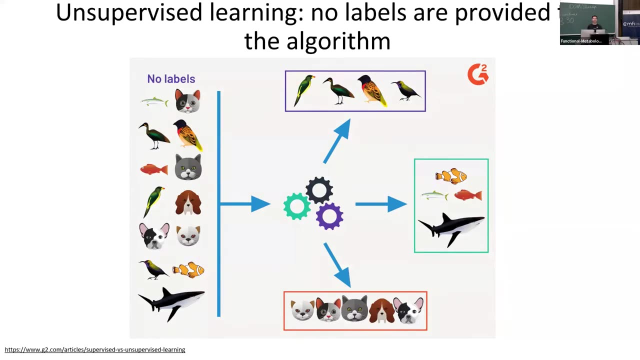 These are just some examples, like random forest probes, the most common used metabolomics, I think, together with some others, renal regression, logistic regression, boosting models and so on. But today I want to focus a lot on non-supervised learning, so no labels are provided. 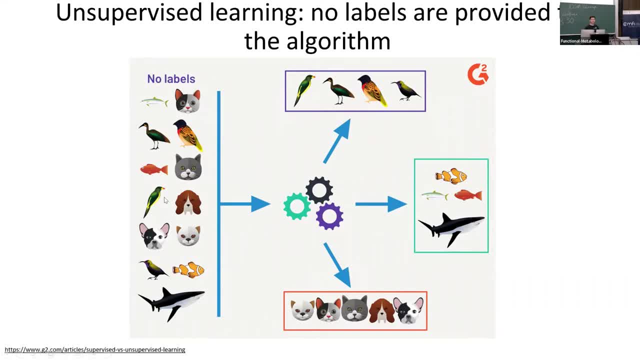 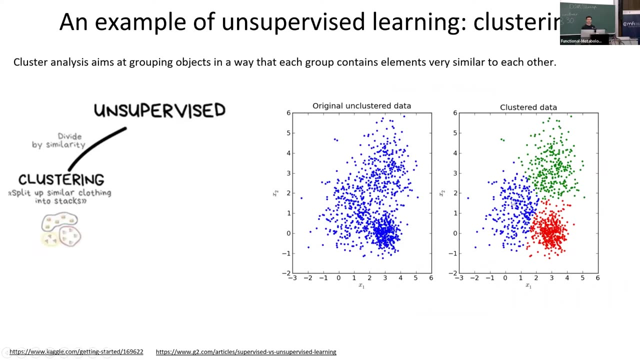 In this case we have a bunch of animals and we want to build a model that will group together objects, observations that are very similar to each other. So here we have the original clustering data and here we have clustering data. So many observations close to each other would be very 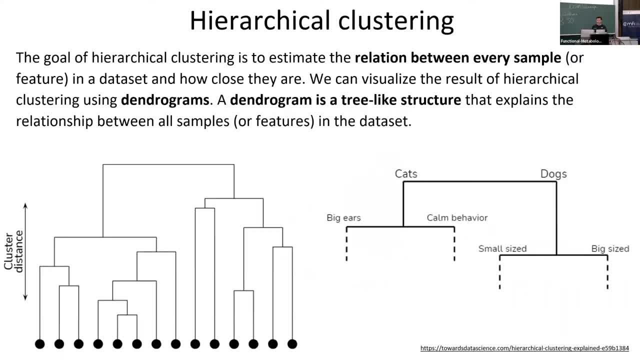 similar in the grouping, And the only clustering approach I'm talking about today is hierarchical structure clustering where basically the goal is to estimate the relation between every sample or feature in a dataset, and it can be visualized in this very nice way with a dendrogram that. 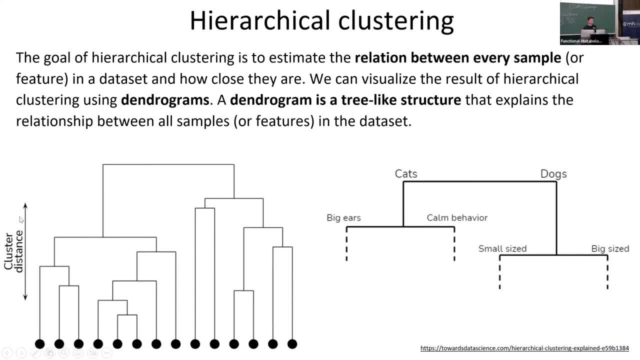 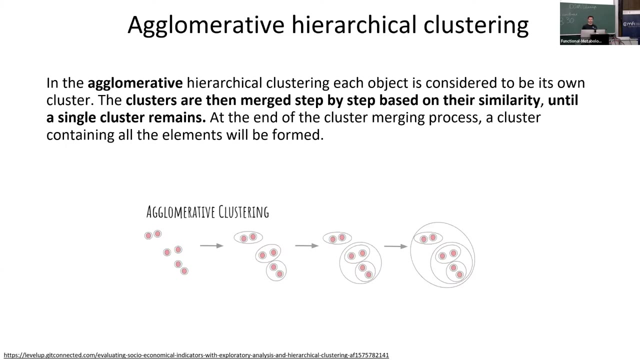 you probably saw many, many times before where the height here indicates the clustered distance. So from the bottom up you have more similar objects until the top, And for instance here we can split cats and dogs and the size and so on. There are many ways of doing it. The most popular is called agglomerative hierarchical clustering. 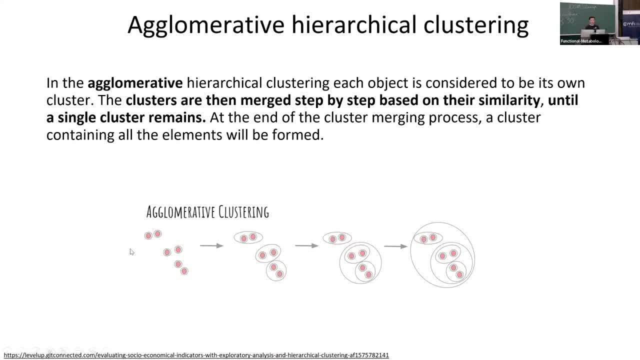 where you have an iterative process where, at the beginning, every observation is a cluster. So every sample, let's say, is a cluster and every sample is a cluster, and every observation is a cluster. And then in our iterative process, step by step, we merge the clusters close to each other. 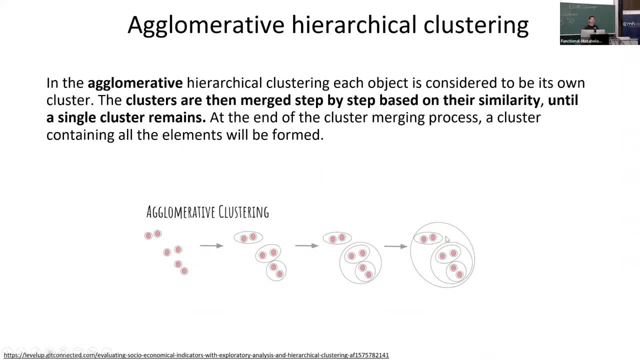 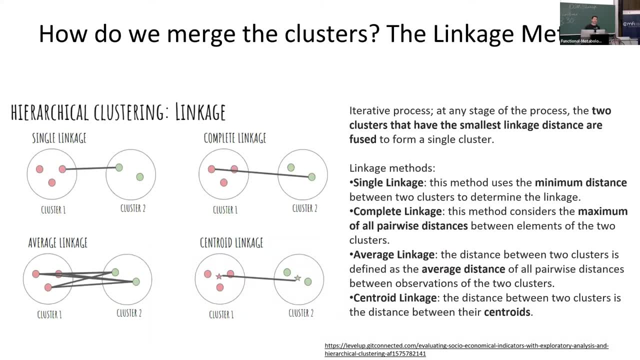 according to the similarities, until this process stops when you have one large cluster. And now we merge the clusters using this linkage method. So you can do it in four different ways. You can calculate the distance between two clusters. that is minimum, or the maximum distance. 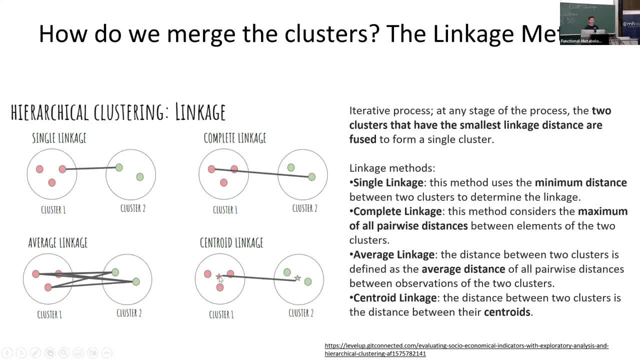 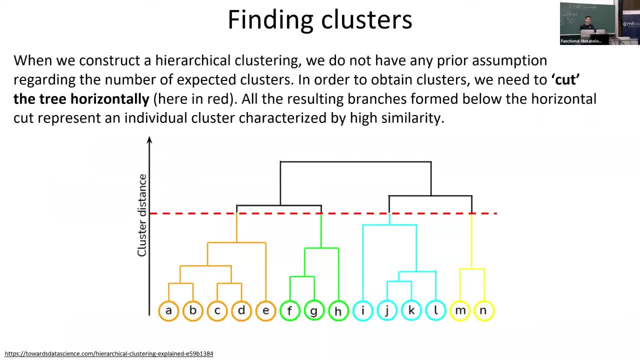 or the average or the centroid distance, And you can also use this linkage method to calculate the distance. So in this case let's say the centroid is the center of the cluster. What we are interested in is to find clusters right And a priori we don't have a defined 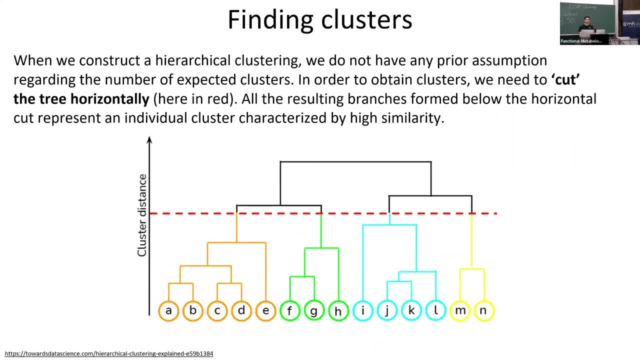 number of clusters when we have a dendrogram after hierarchical clustering. So we want to cut the branches of these three at a certain height where it's for us meaningful. And this is quite challenging because it can be quite dependent on your field. the samples that you have: 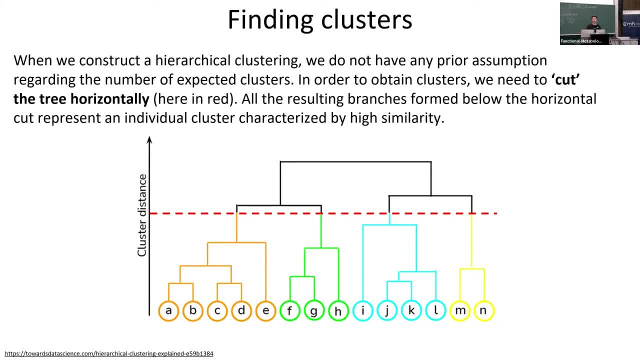 the visual inspection that you do in your data, but it can also be computationally calculated and we will show you in a moment. So here, this dashed line indicates where I cut the tree and all the branches. below are the clusters that we've formed. There are different ways of cutting the trees. 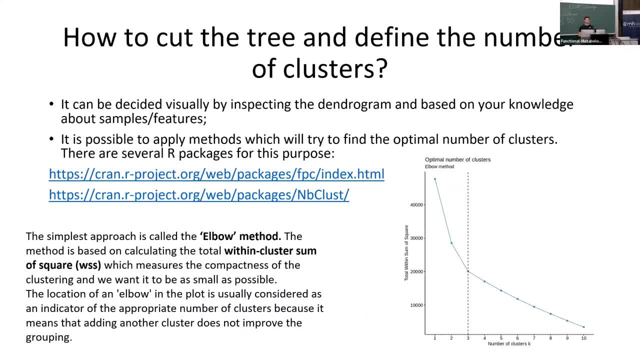 One of the simplest method is called elbow method, where the within clusters sum of distances is calculated every time a cluster is merged together and you can plot this and where you observe in this curve a bend, a knee some people call it, or an elbow is the proper amount. 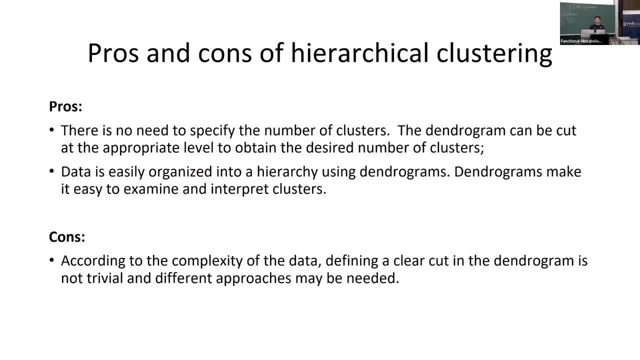 of clusters. There are pros and cons of hierarchical clustering. The pros is that it doesn't need a defined cluster. you can just plot the dendrogram and expect the data. but can also be very challenging to define a cut in the dendrogram if you are 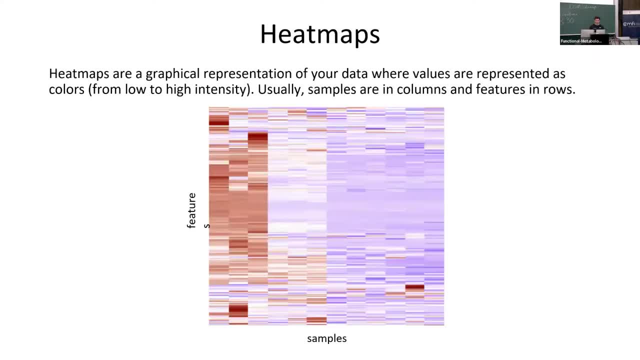 interested in defining the number of clusters, Probably also very used to heatmap concept. heatmap is just a visual visualization of your data, your samples here index and features. The color is just the intensity of your values, in our case the intensities of the metabolites. 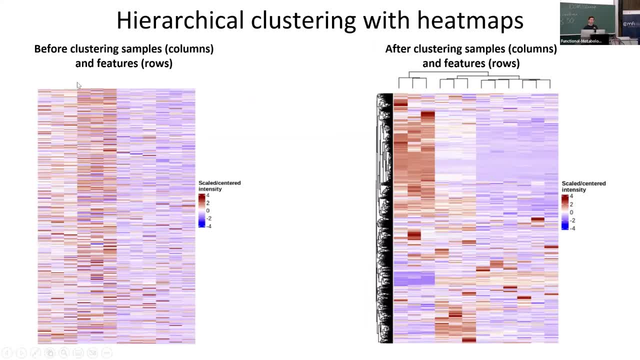 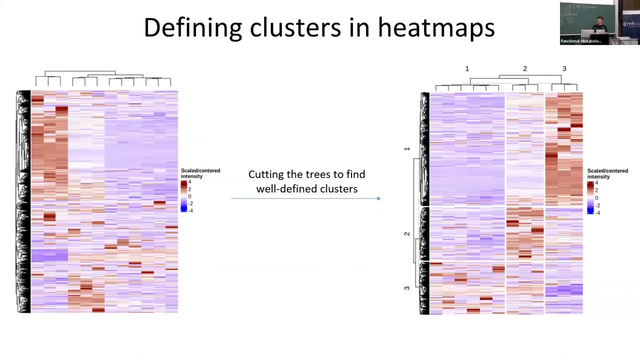 Here you can see a heatmap before doing hierarchical clustering. so there is no order here and here on the right you can see after hierarchical clustering. As you can see, the rows and the columns are reordered according to the most similar objects or observations. Next slide: 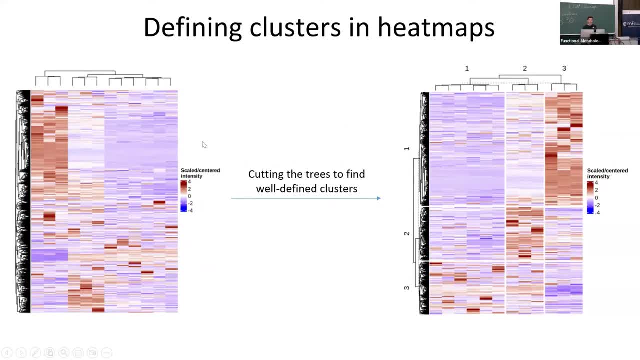 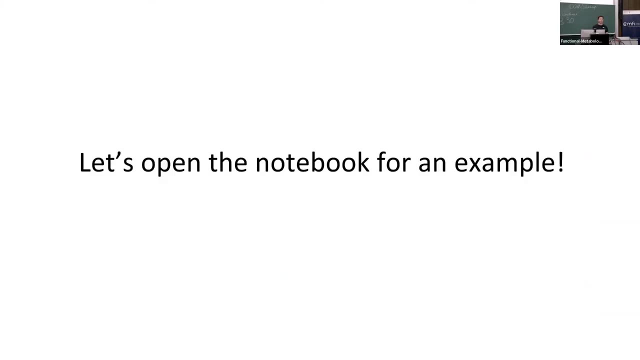 And we can define the number of clusters in the heatmap itself by cutting the tree, as I showed before. And here you can see three main clusters according to the samples and three main clusters according to the features. Okay, so let's come back to the notebook. 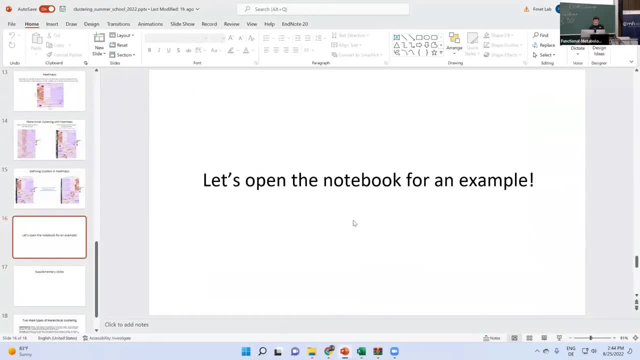 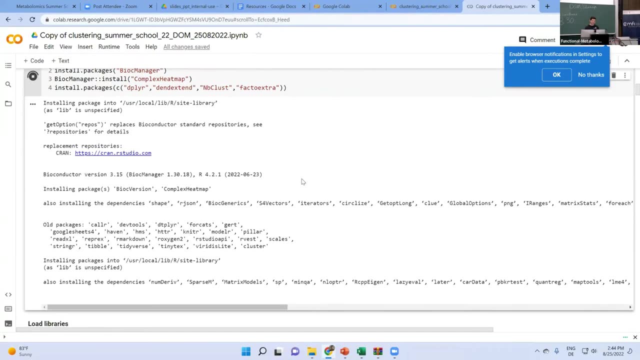 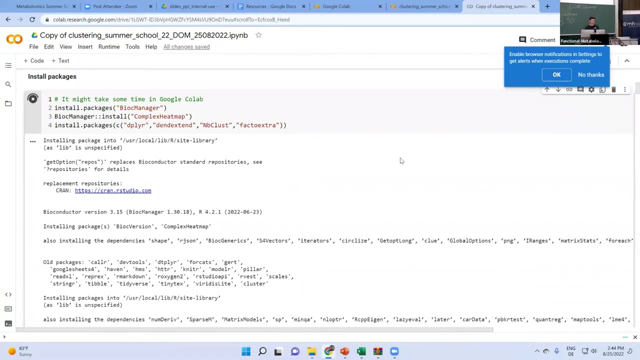 Let me know if there is anything unclear. of course, My strategy didn't work. I hope that coming back here you could have fixed it- Maybe that's the other question in the meantime. So the clustering: you built a dendrogram first and then plotted for. basically. 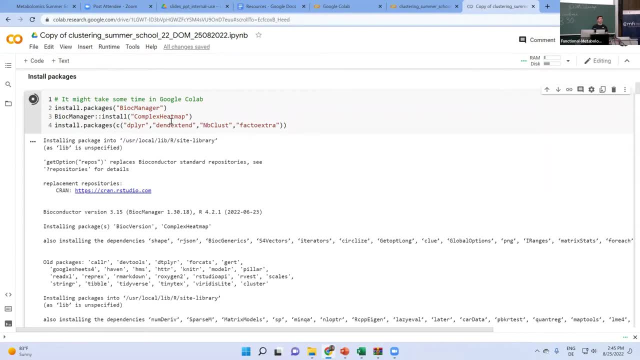 Yes, But at least in phylogenetics, there are many, many different ways to build a dendrogram, Sometimes with quite different results. That must be the case with this stuff as well. So even when we run the code, actually every time there is some sort of stochasticity. so 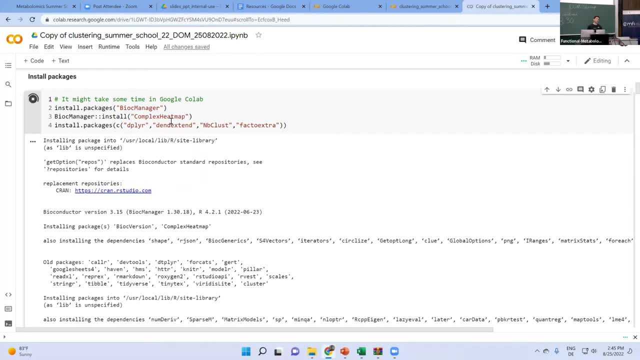 every time you generate it could be different according to the complexity of the data set. So that's why we fix usually a specific point in the code that we will show and you say: I want reproducible results, So every time you will generate it will be the same result. 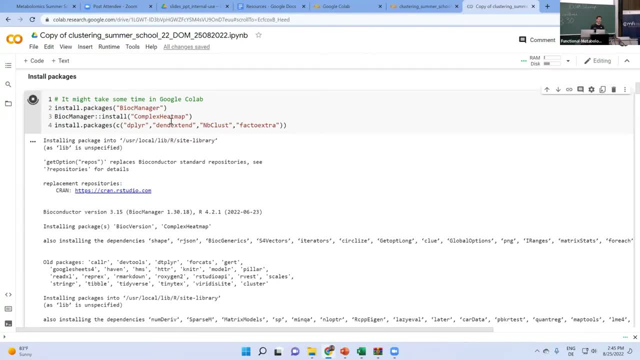 But there are different ways of cutting the tree is true, In phylogeny you use PGA or something like that, I think, or something I don't remember. Yeah, Some different ways, And the hierarchical clustering is just one of the most basic way of doing clustering. 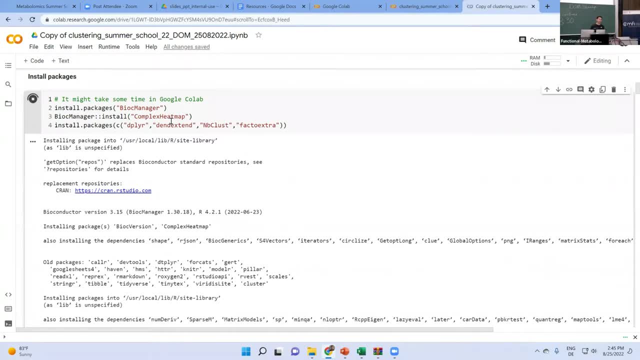 There are many others, like amines or density clustering and so on, that are more advanced, But it's the easiest to explain, I think from the pedagogical point of view, because as a visual You have your representation or your samples and it can become very difficult to interpret. 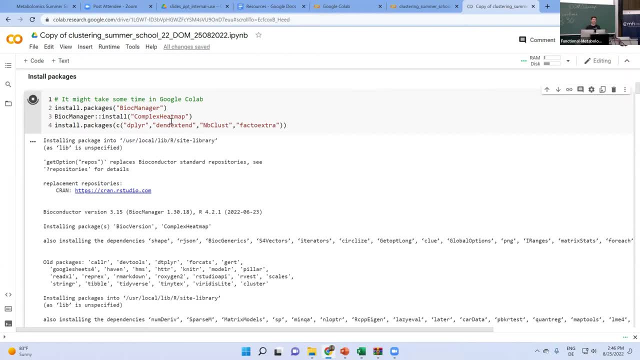 when you have 2,000, 3,000 samples, of course, Or if you plot the features, then it would be 5,000 features and every line in the tree is a feature. In the end, the question is, is it a meaningful clustering? 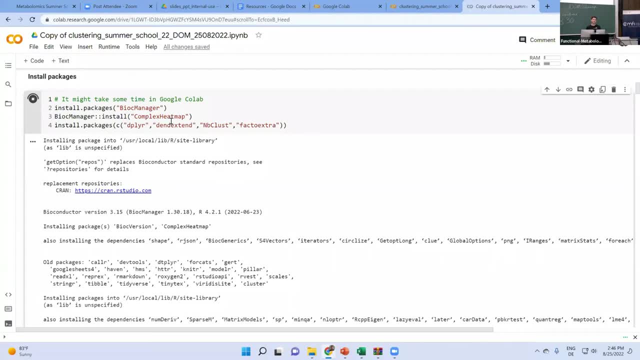 Yeah, to do that- and there are some comments here- you have to check for the stability of the clusters. So there are methods. You have to shuffle around the labels, for instance of the samples, and verify if your clustering was robust or not. In that case you can refuse the clusters or not. 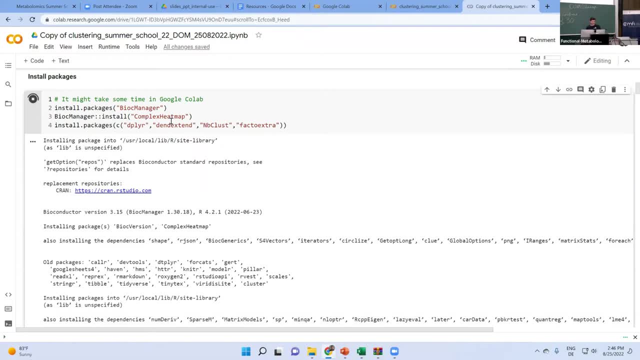 We need an elevator song here. Yeah, it could be. Yeah, Are yours done? Yeah, Depends on the map, Of course, you can go for coffee or whatever instead of inside. Yeah, Now we will upload our files. Yeah, I think we have a lot of time. 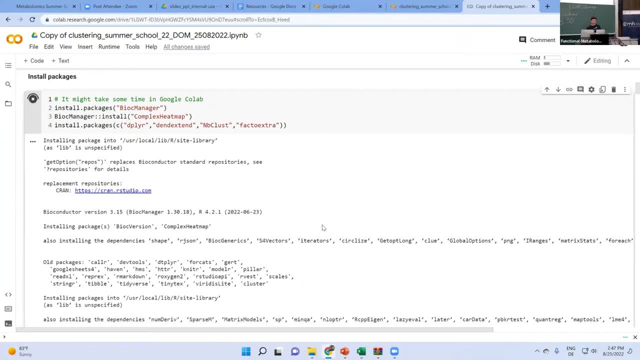 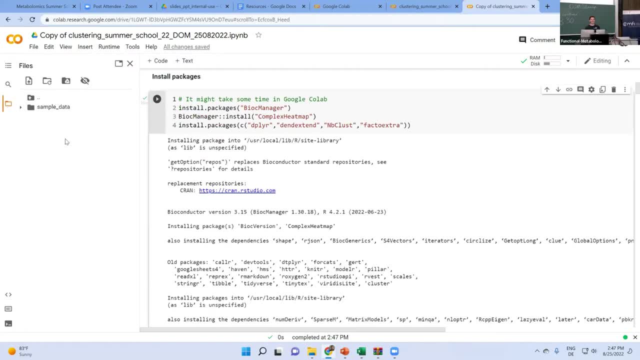 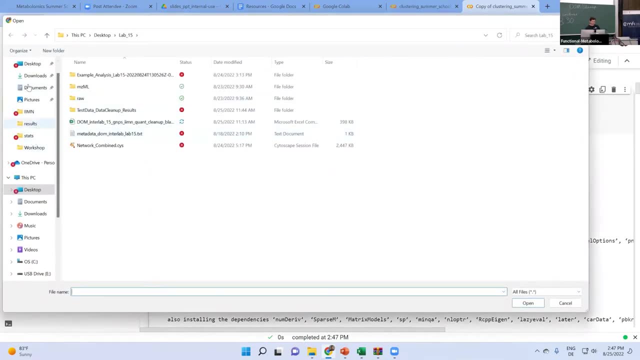 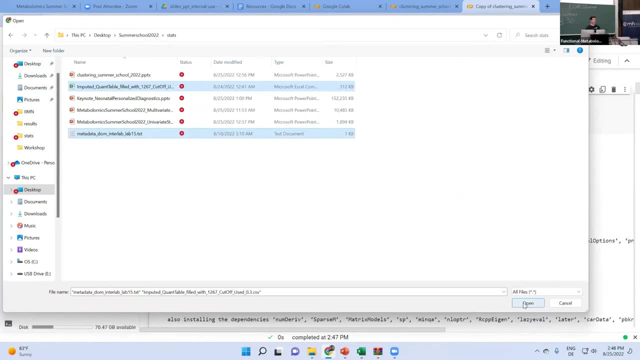 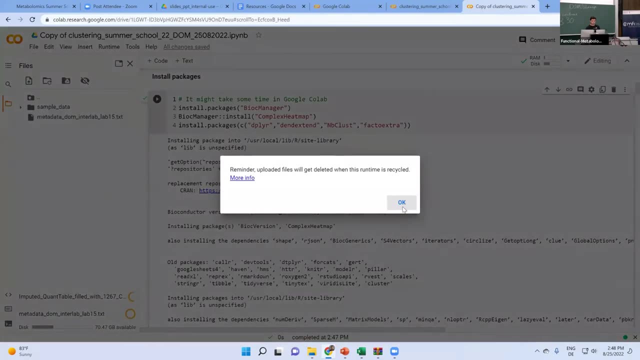 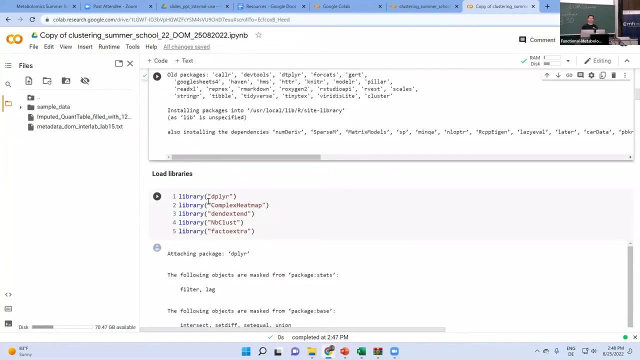 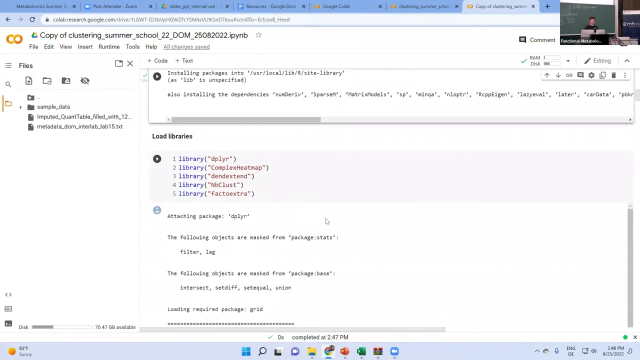 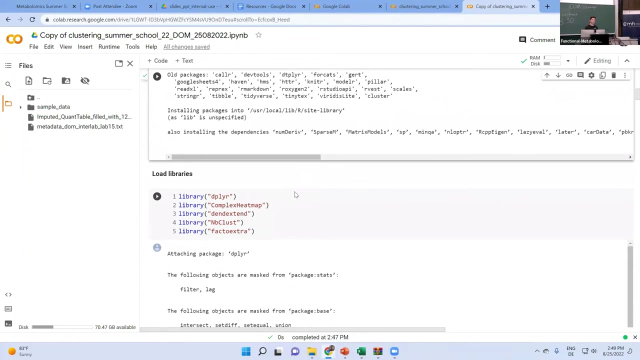 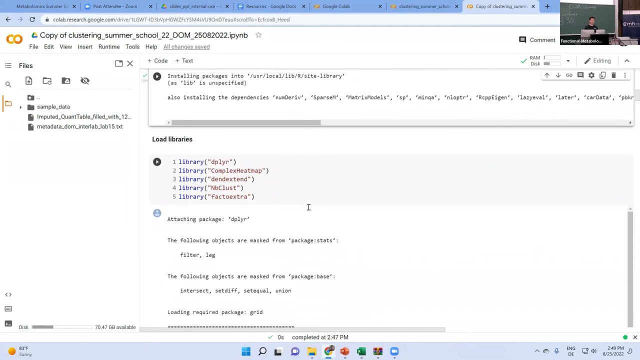 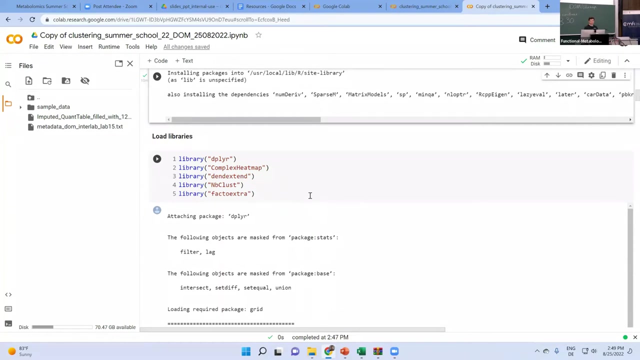 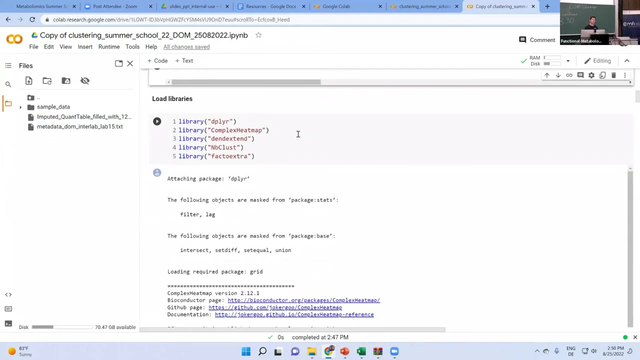 The imputed quantification table. Yeah, the same input as the PQA. Are you all in? Okay, wait, Okay. Okay, Did you install the libraries? Yeah, everything's down. Libraries are done. Nice, Okay, Does it work? 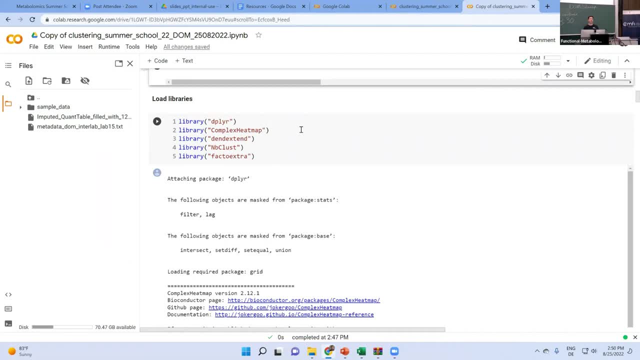 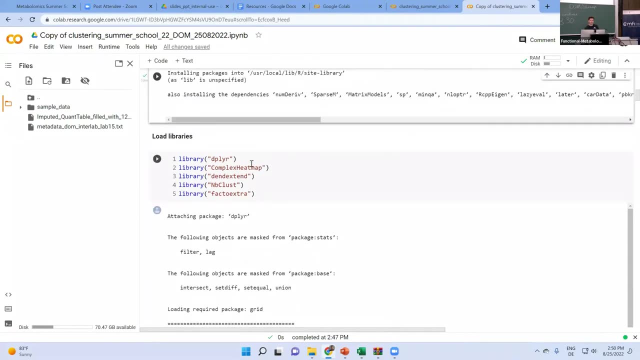 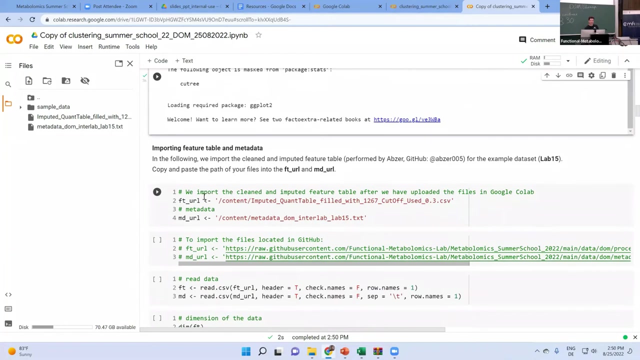 Yeah, Yeah, Install all of you. Yeah, So I'm moving on, okay, So first we load the libraries- This time should be fast- And then here you can just copy and paste the path for your files, as before, if you remember. 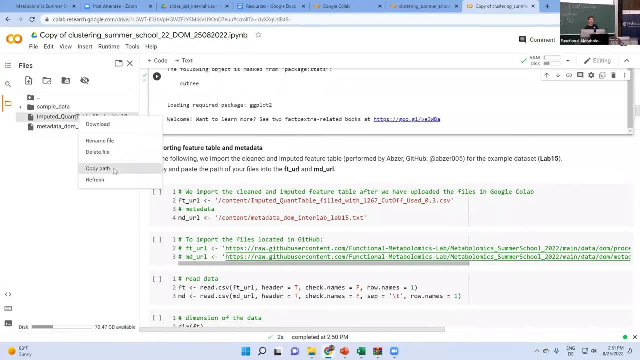 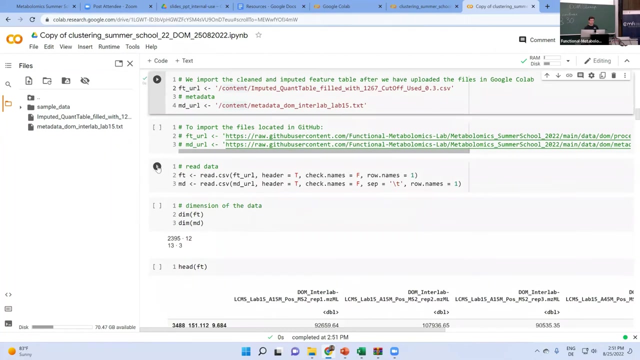 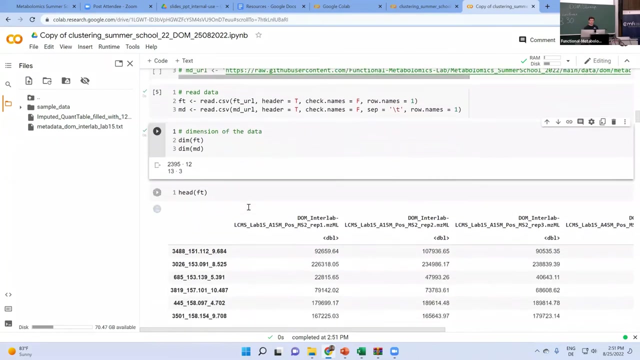 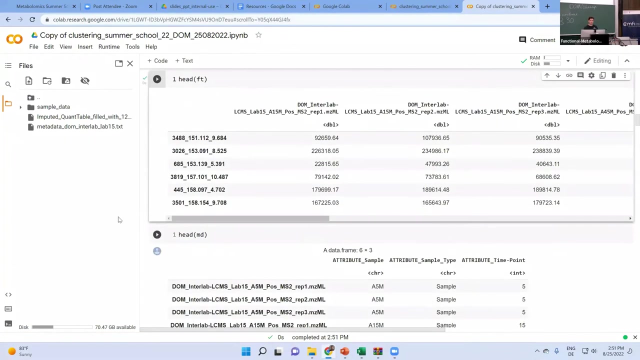 You can just do like that and copy the path, Yeah, And then you can put it here, One for the feature table and one for the metadata file. Then we will read the data and we'll check the dimension of our files. We can visualize, as you know already, the first six lines of our feature table and the first six lines of the metadata. 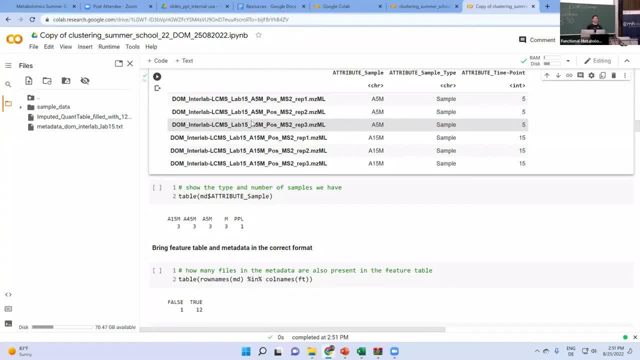 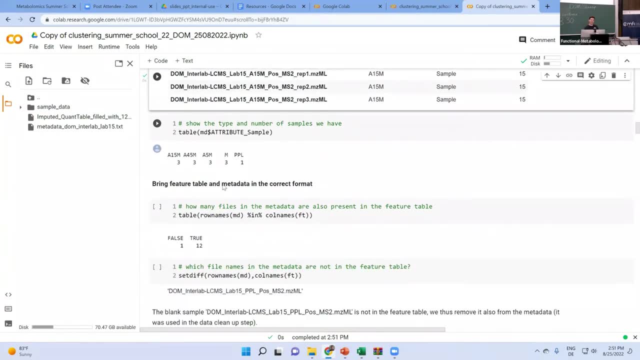 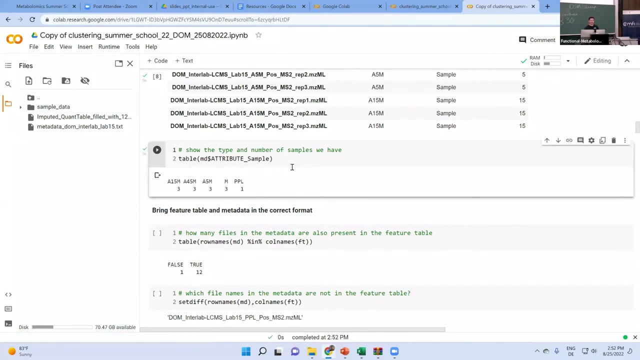 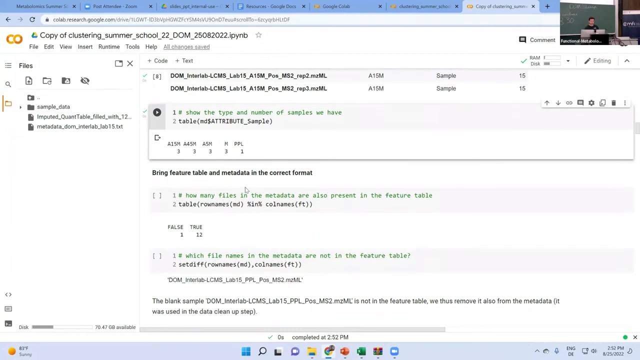 Did you manage to read the files? Yeah, No issues. Okay, good, Wonderful, Wow, that's a first time. This is just to check what are the attributes of our metadata, the attribute sample. As you can see, we have one paper blank still. 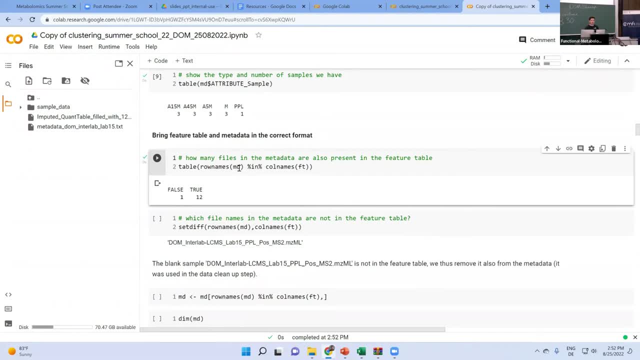 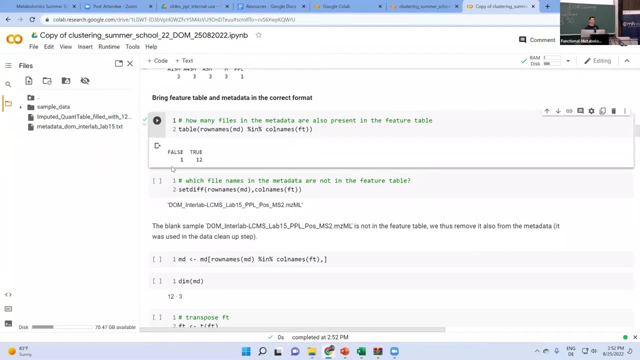 And this is to check how many of the samples in the metadata are in the feature table. As you can see, one is not and it's the paper blank. So we are going to check this. You can see the paper blank here. 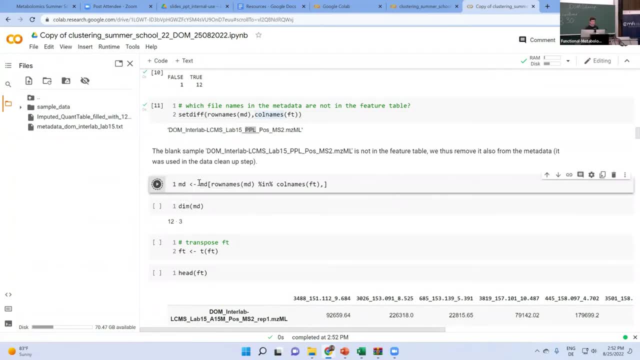 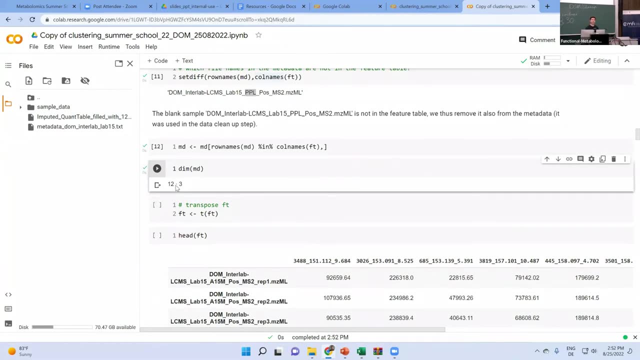 We want to remove this from the metadata And we check the dimension again. So you should have 12 samples right, And three columns. We transpose the feature table because we want the features in the columns in our analysis And we check again. 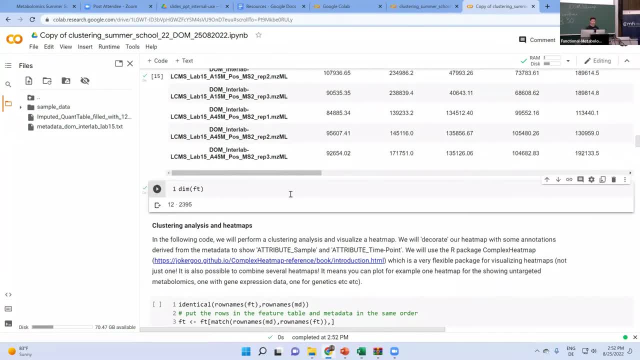 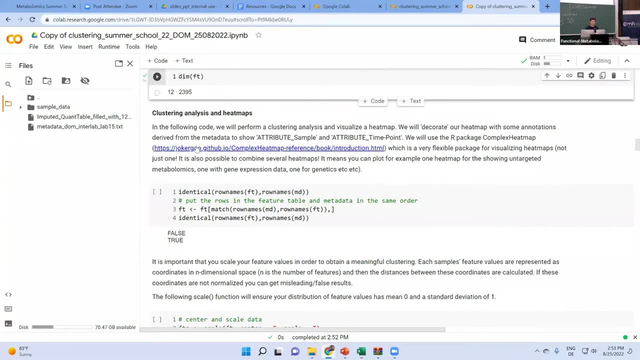 Yeah, You check again the dimension if you want, And it should be like 12 samples and a specific amount of features. We check if the rows are in the same order. At the beginning they are not, But we transform them to be in the same order. 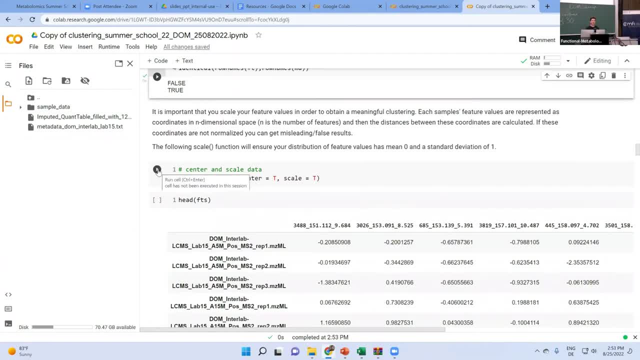 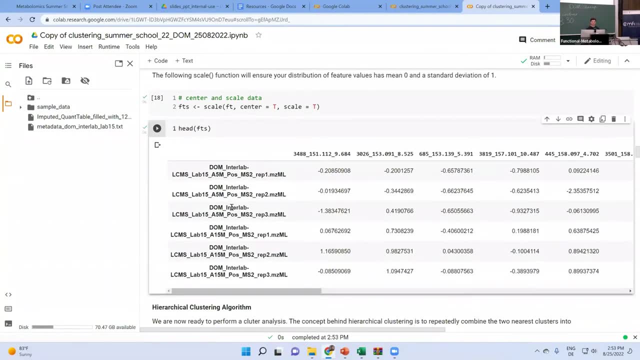 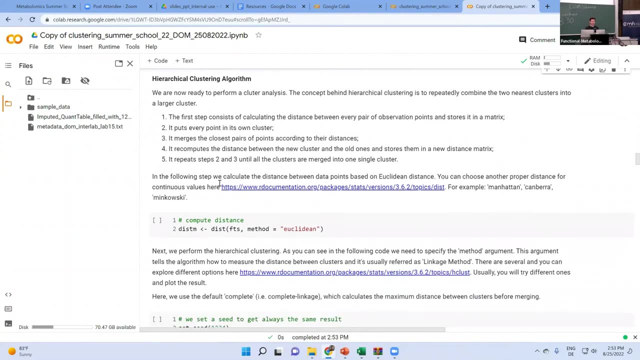 We scale the data. All these steps are the same on the peak array. if you have a DejaVu, Yeah, And then we check again. So here it starts the actual clustering. I reported here again the steps, But we don't need to go through that again. 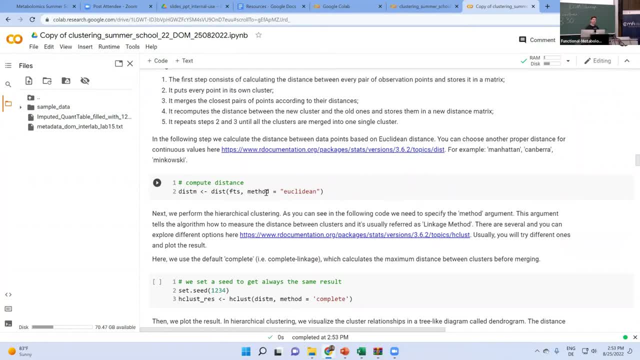 There are different ways of doing it. There are different distance matrices, as Madeleine already mentioned Here. we will go with Euclidean, but you can change it with Canberra, You can play around with it, And I reported also where you can find all the distances that you can put. 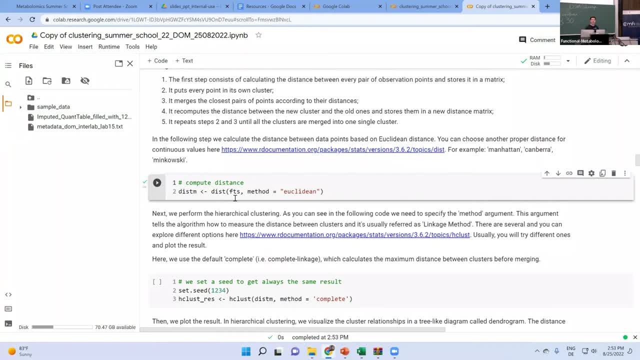 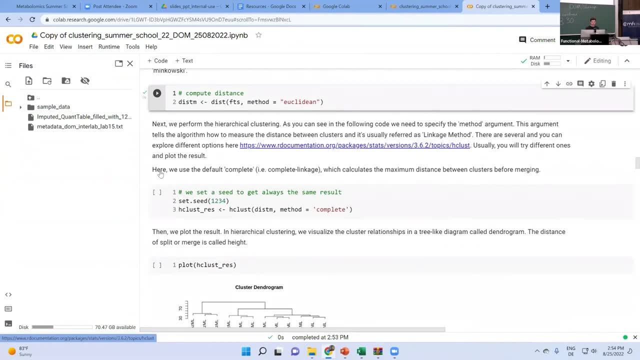 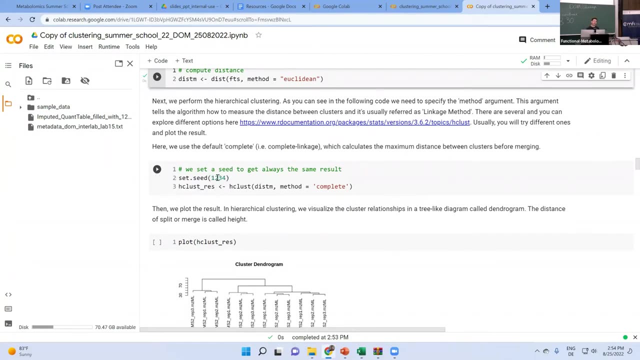 So we calculate first the distance, The pairwise distance, between all the samples, the features and samples, And here we calculate the hierarchical clustering, As I mentioned to you before. here we set this seed. that is just a way to produce the analysis, Always in the same way. 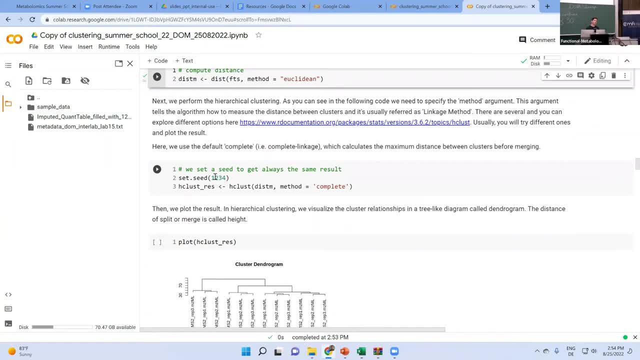 If you don't put this, then the result can change, because it's stochastic, And this is just one of the methods that I mentioned: The linkage method. It can be complete, It can be average, It can be centroid. So if you want to do something similar to bootstrapping, you would do hundreds of different things. 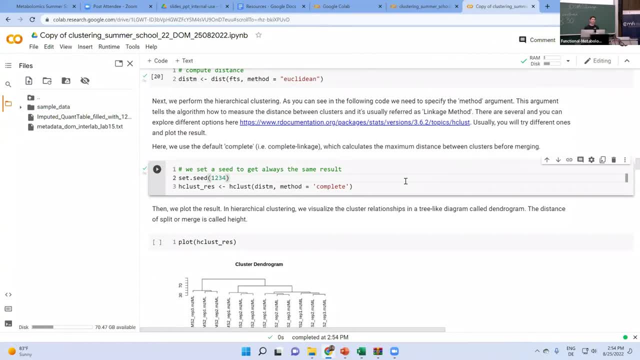 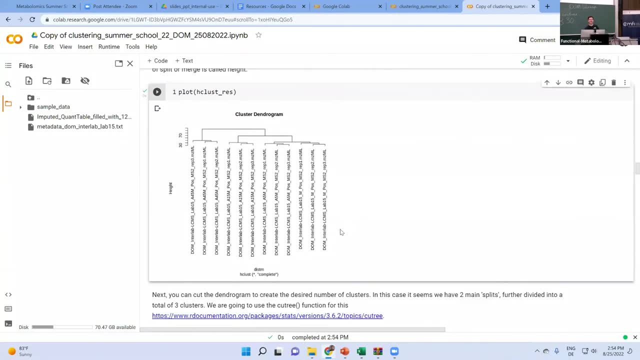 Yes, exactly, And shuffling the labels as well. Then we plot. Now I'm curious to see if you get something similar or something completely out of the blue. So what I get is that the sample, The samples 45M, cluster in a way together in this split. 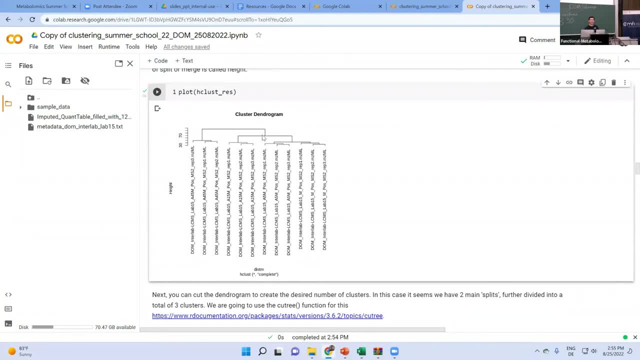 I don't know if you get something similar. And then there is a second split here, Major split, And in this major split we have some two sub-clusters- we can call them The 15 here, And the M and the 5M. 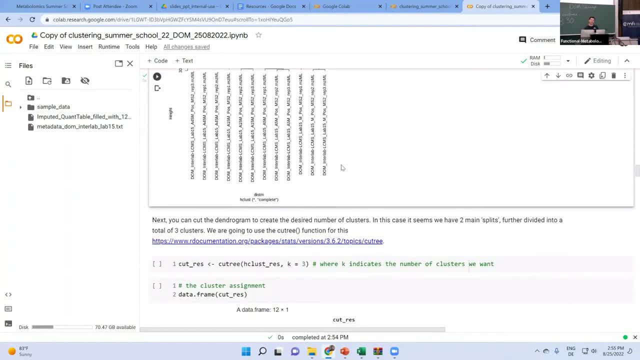 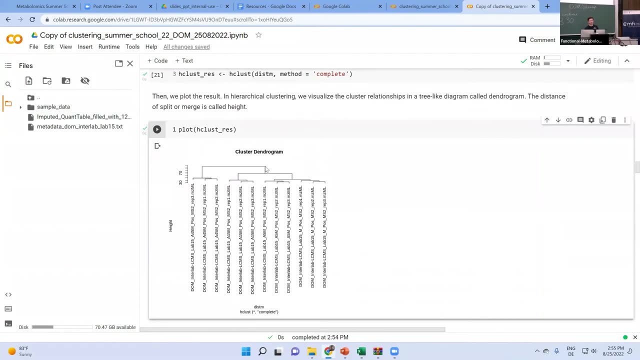 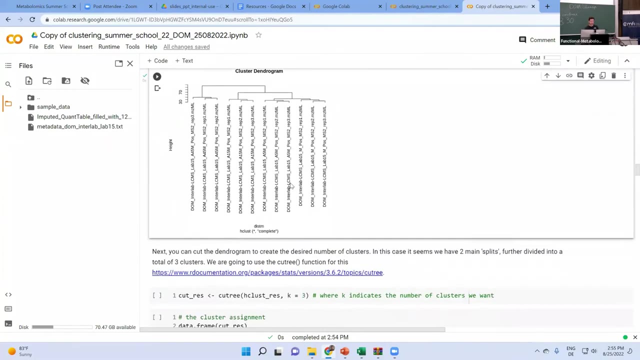 You get something similar, Good, Reproducible, We can publish it. Next, it seems here that there are two main groups, But it seems there are other two sub-clusters, So we want to cut the tree, And in this case this parameter indicates how many splits we want. 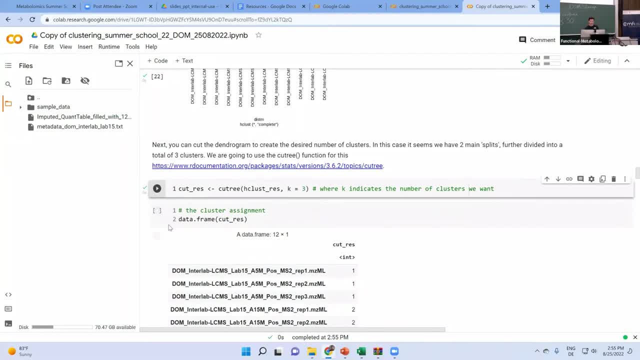 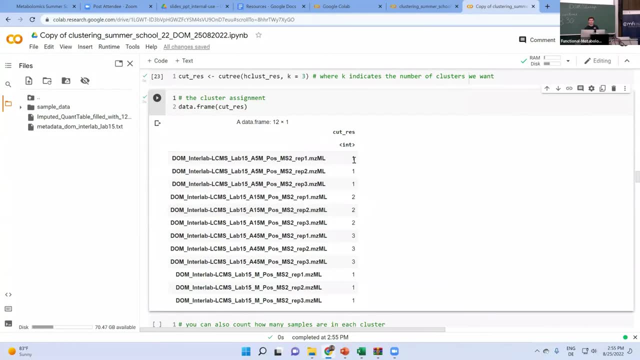 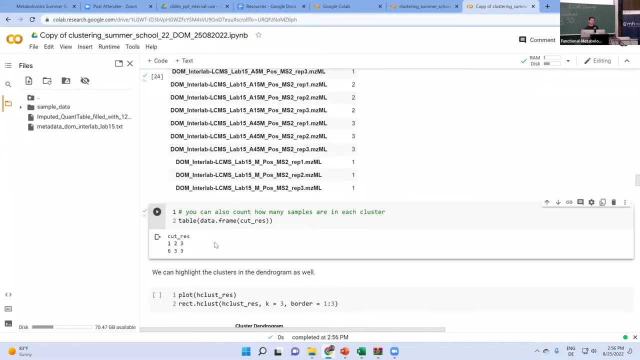 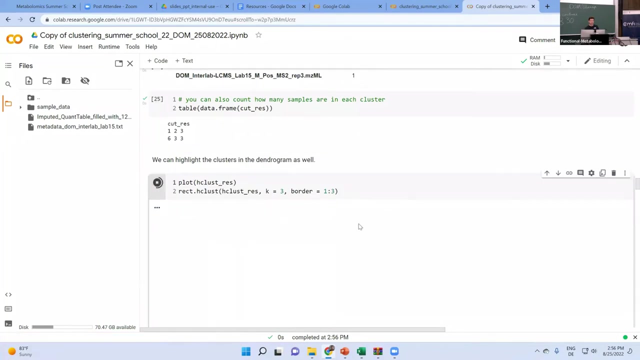 So in this case I say three And we can check the result. Which samples belong to which cluster Is it clear? And you can check how many samples are in each cluster. Then we can also highlight with the colorful rectangles the clusters. 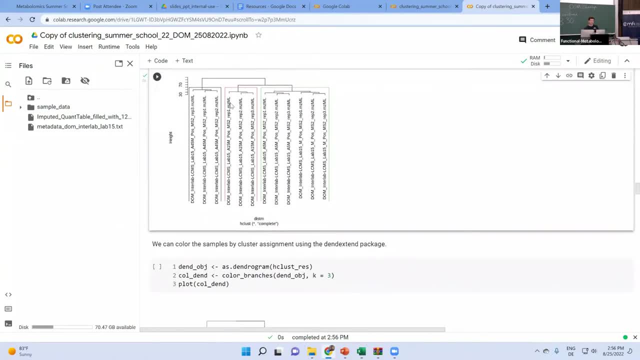 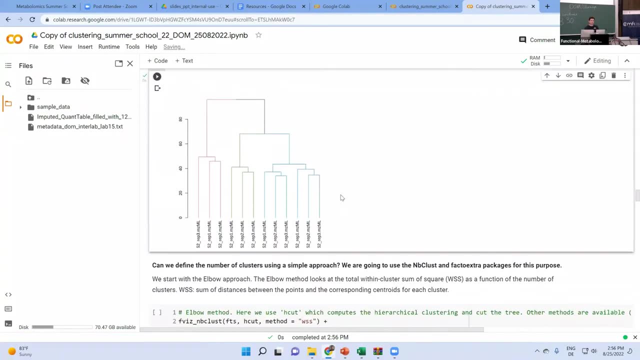 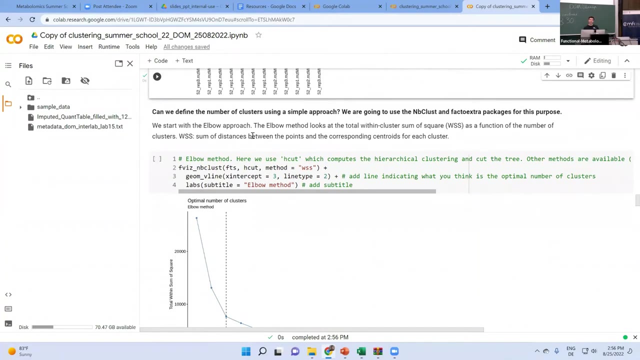 If you want to use it for publication or anything else, As you can see here, And you can also color the branches if you like. As I said, it can be tricky to define the number of clusters. Now I say three, But we don't really know very well at the moment. 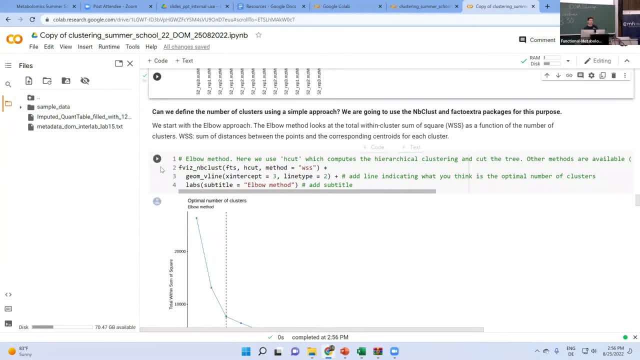 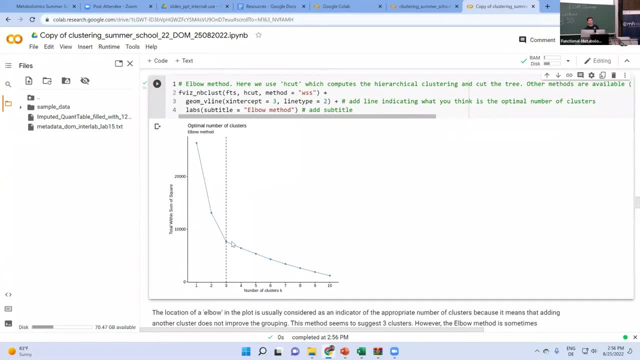 Therefore, we will proceed with this elbow method that I mentioned in the presentation. Let's run this And we can see this: bend This knee here, Or elbow At three. So it could be that there are three clusters, But the elbow method is a bit sometimes ambiguous. 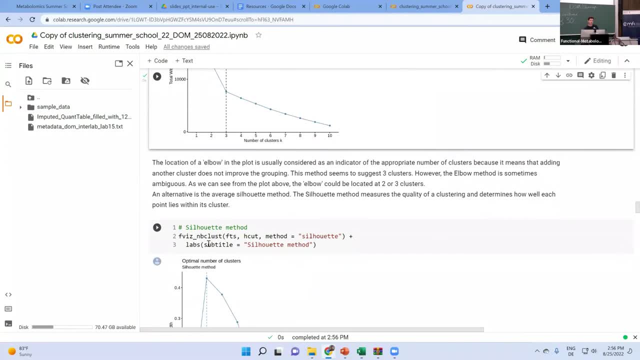 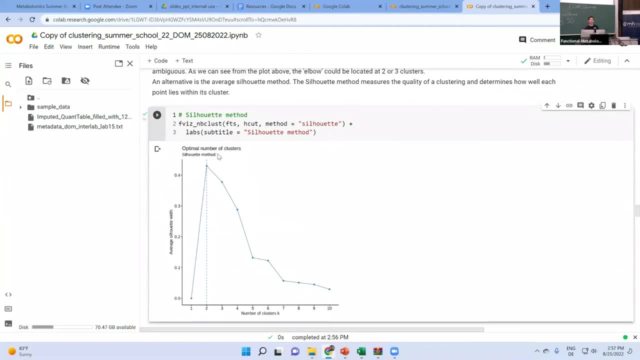 It can be two or it can be three. Therefore, we will perform another analysis, And it's called silhouette method, And we will check how many clusters suggest this. In this case it says two, Because there are two main splits actually. 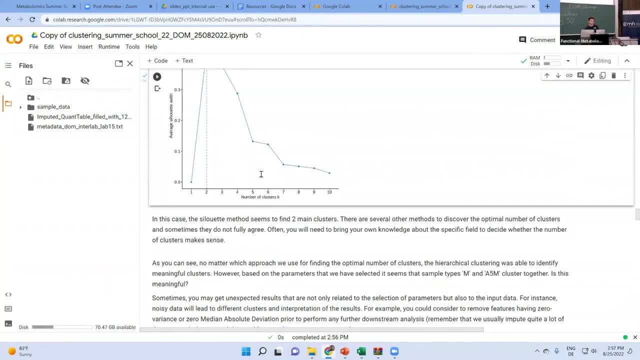 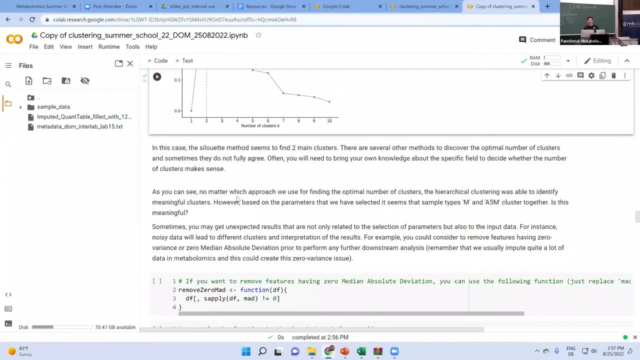 You get something similar, Yeah. Another thing that it could be Altering your analysis in the clustering If you get something completely different Is the input data. Sometimes metabolomics data are very noisy. We impute a lot And we create this zero variance problem. 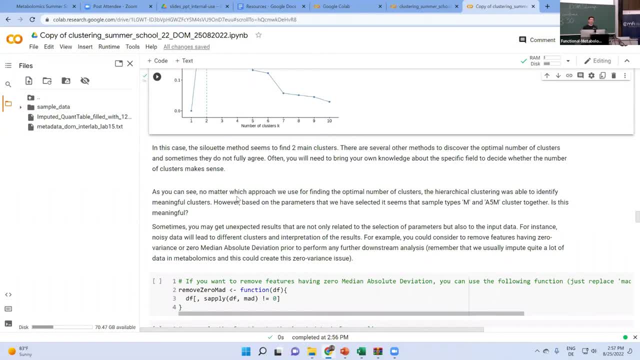 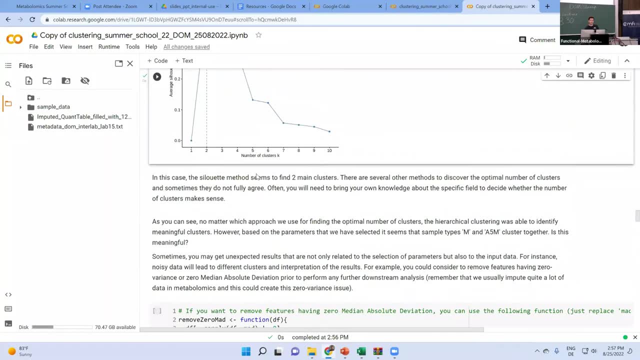 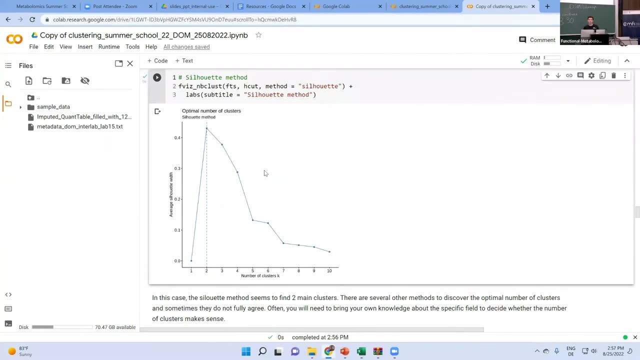 So imagine zero, zero, zero, zero And one feature that has a value. So let's see what happens if we remove those features. Sorry, Can you go up? Yes, It's different. How many clusters suggest this? I have one, two, three. 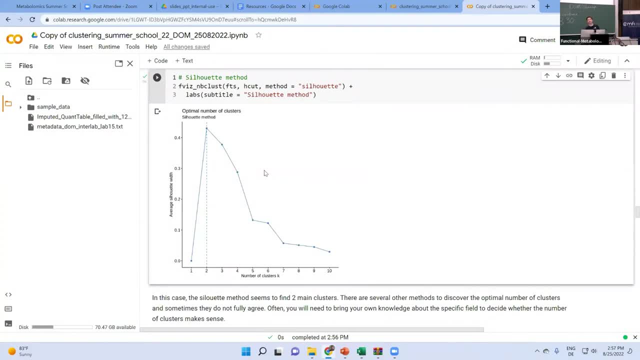 Three clusters And the elbow method as well. Yeah, Oh, that's nice, They agree. So what if your clustering suggestion is clearly wrong? Yeah, Clearly wrong. The PCA gave the clustering, as I would expect. Yes, Yeah, Exactly. 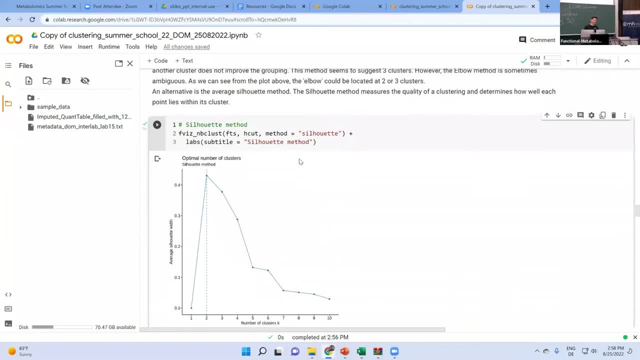 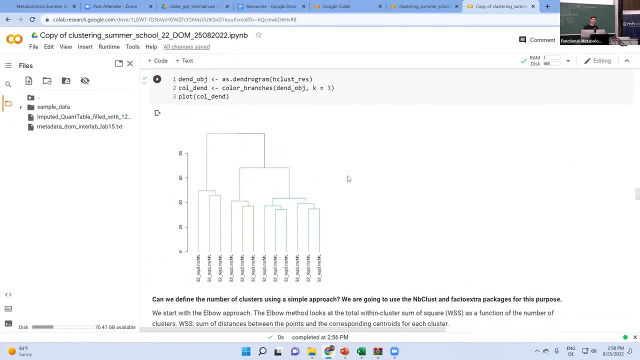 Because the interpretation from the hierarchical clustering it's not 100% what you expect as a cluster. It's more a visual interpretation of the hierarchical relationship of the groups. So I will use more advanced methods, like a means or density clustering, to discover more meaningful clusters. 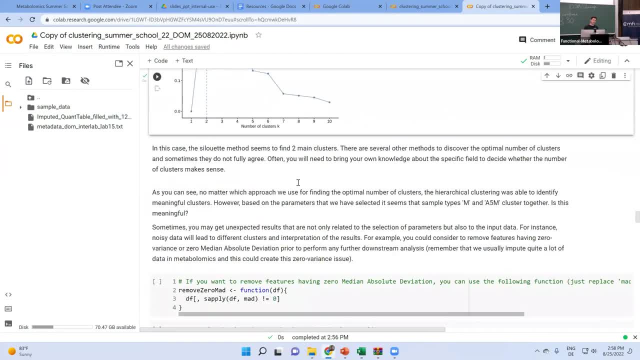 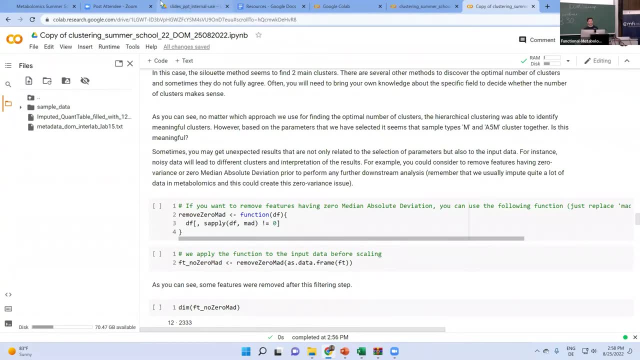 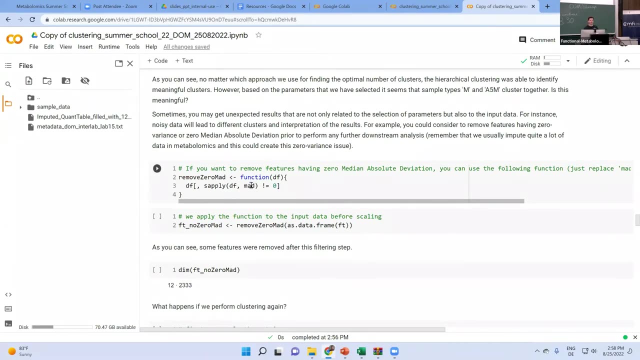 But also, as I wanted to mention here, Sometimes it could be because you have this zero variance problem And then when you cluster, you obtain things that are unexpected. So I wanted to show you what happens if we remove those. In this case, I don't want features that have zero median absolute deviation. 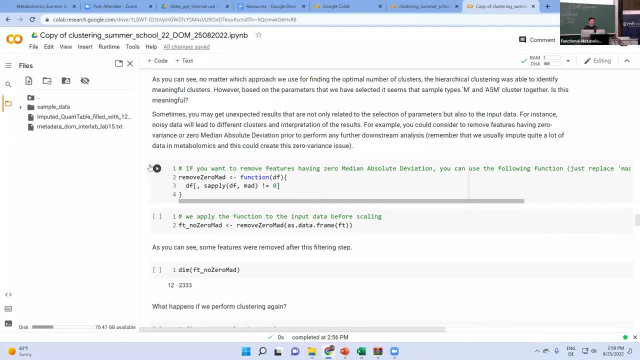 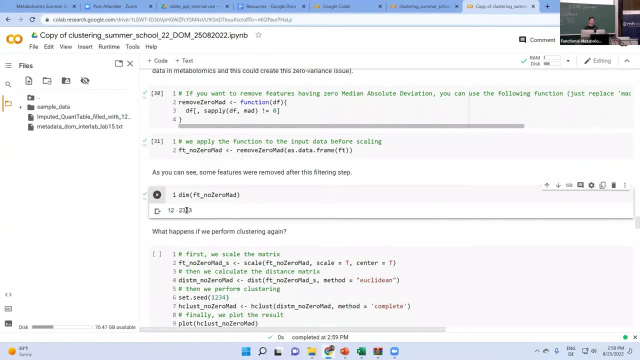 Let's say variance. You can change this as bar, It's the same. Remove this And we check the dimension. In my case, I don't remove that many features, But I heard that some people have 50,000 features. 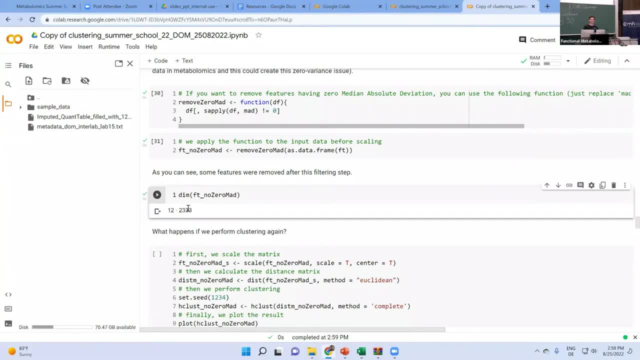 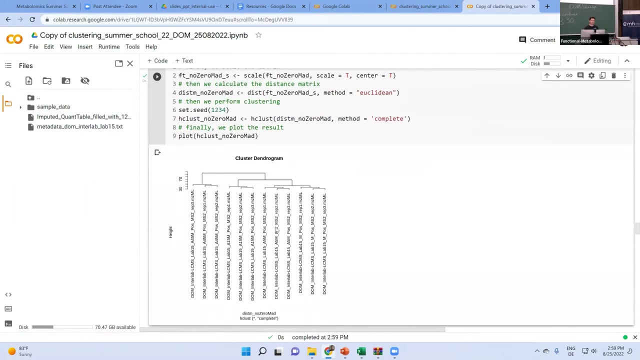 So maybe you will reduce a lot your dimensionality. It happens to you. You remove a lot of very few features, Very few. Okay, So if we generate again the clustering, for me it doesn't change. So I can conclude from here that the samples here 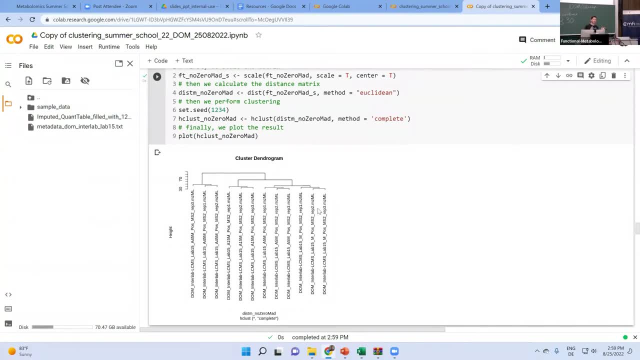 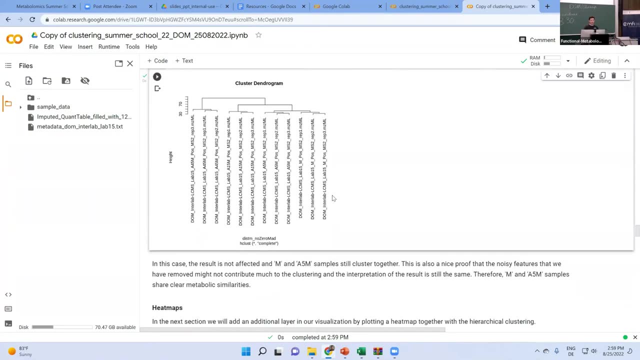 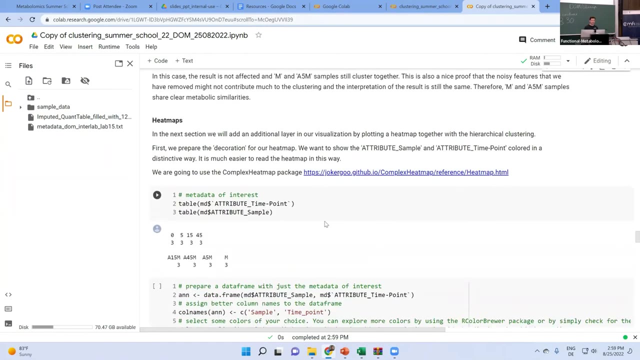 M and 5M actually are quite close And they make sense because in the deletion process they are also close in time. So we excluded that this clustering is biased by the fact that there are many noisy features. Finally, we want to generate the heatmaps. 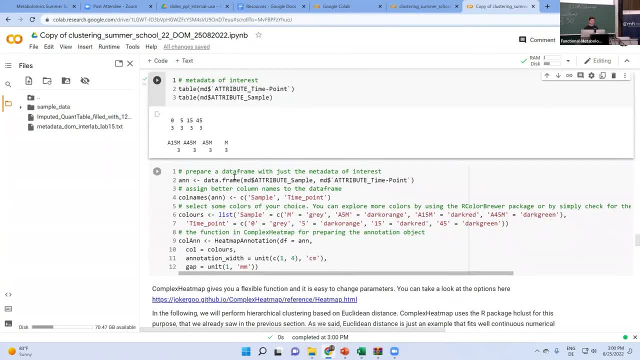 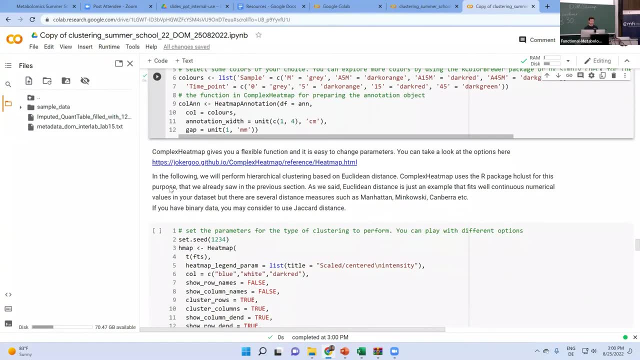 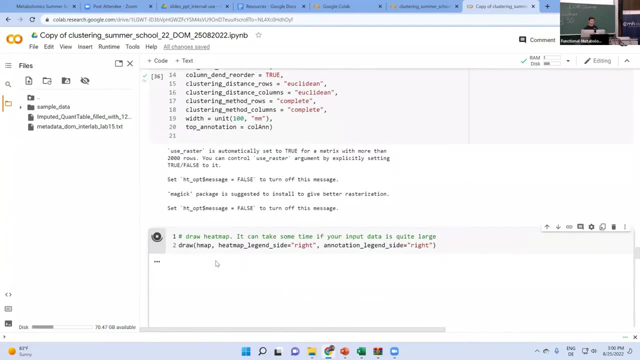 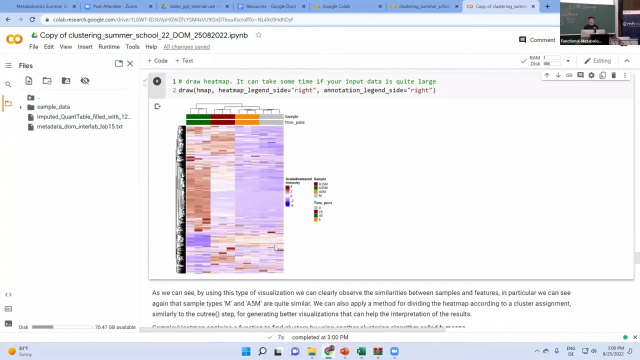 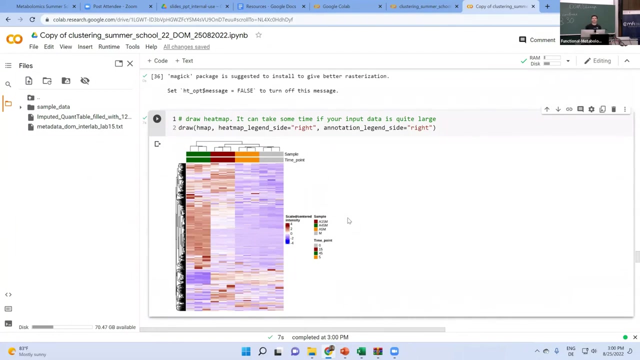 We check again the attributes that we have And we prepare here our input data for the heatmap And then we block. Do you get something like that, Something very different or something very similar? Yes, Somewhat different. Which difference do you see in yours? 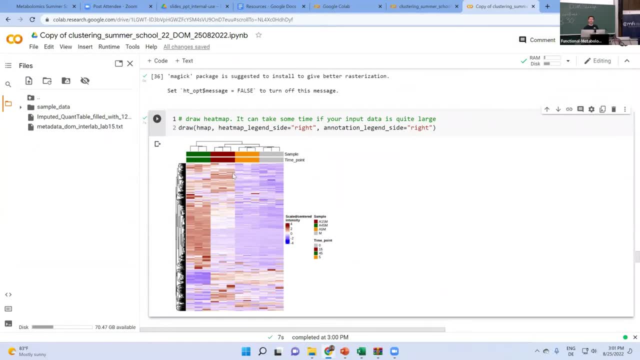 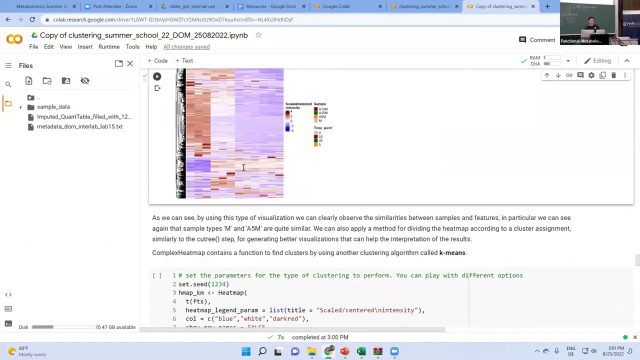 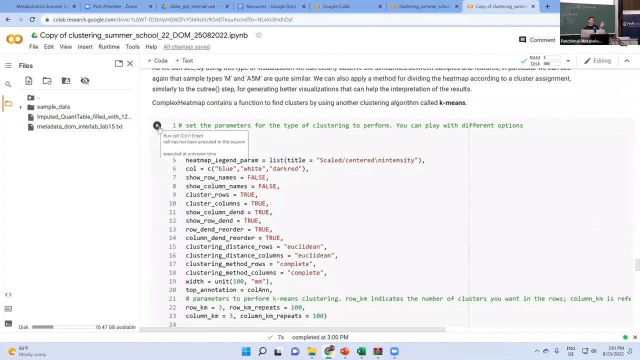 Okay, Yeah, This one could be just when you block, But you can check how the hierarchical clustering is to see if it makes sense. Yeah, And it could be, because also, again, it starts from a random point And, as I said, we can perform a clustering to break in pieces, in blocks, these groups. 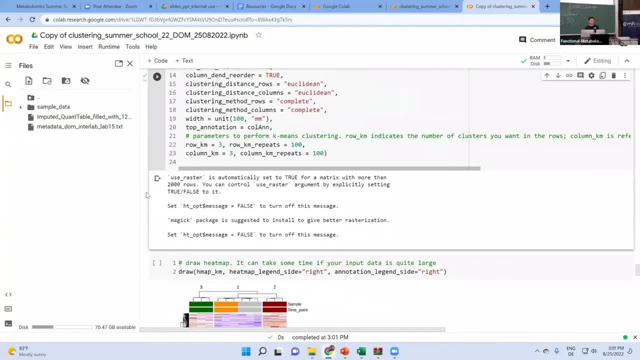 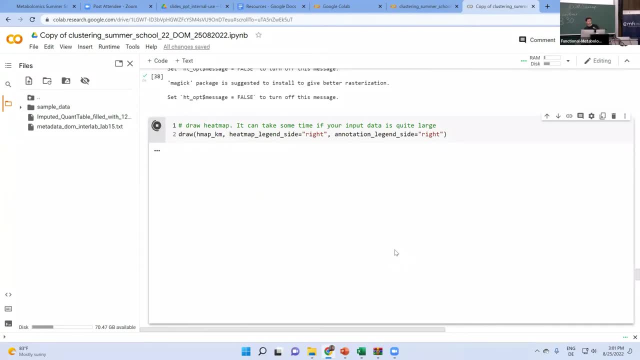 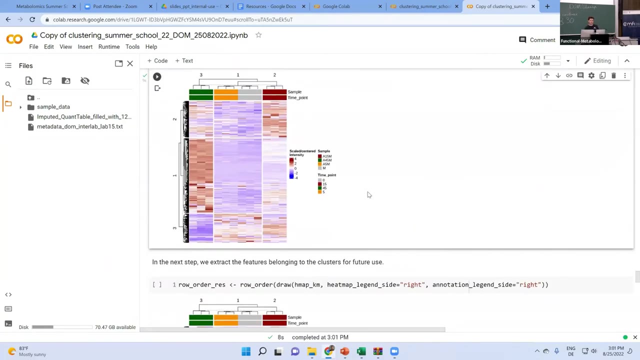 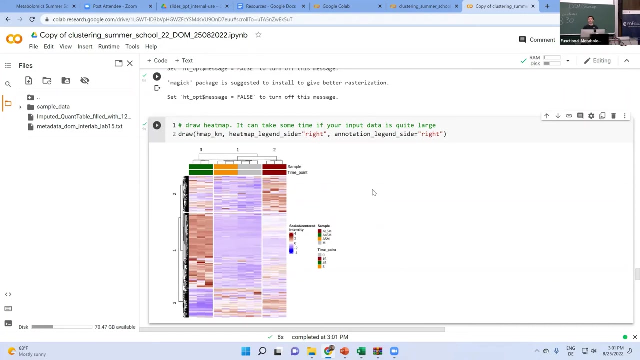 We can cut these trees to obtain clusters And you obtain this nice visualization where you have a clear cut of the groups, As you can see. But I want to underline that this is what I observed in my dataset. But you can play around, of course, with the parameters and say: I don't want three, I want four. 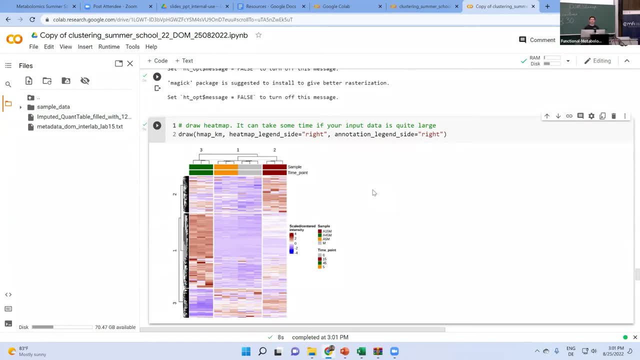 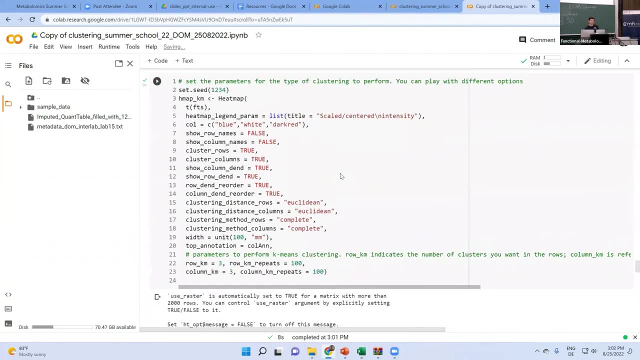 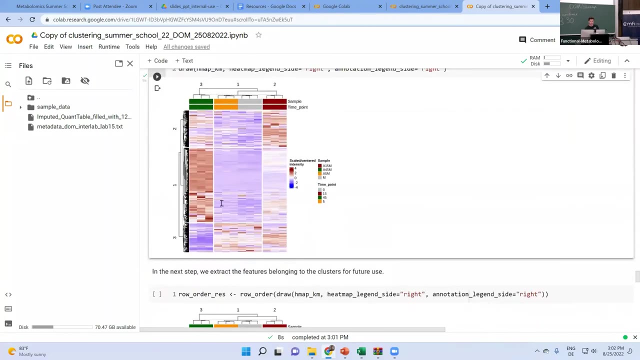 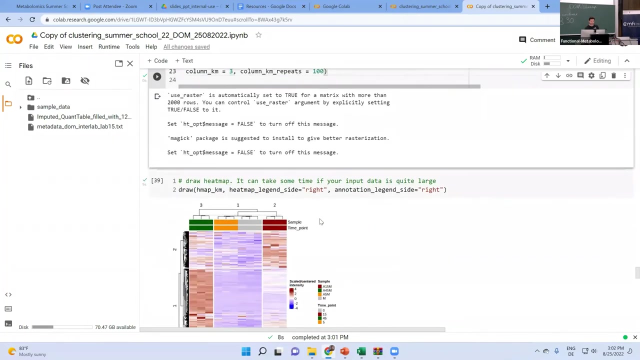 And all of my elbows or silhouette approach, suggest four clusters or three clusters? of course, Yes, Can you please let me change the number of clusters? Yes, In this last part or before. In this last part, you can change it. here for the rows and this is for the columns, and here this is. 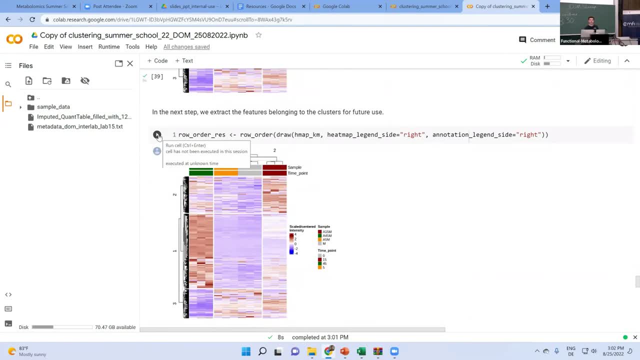 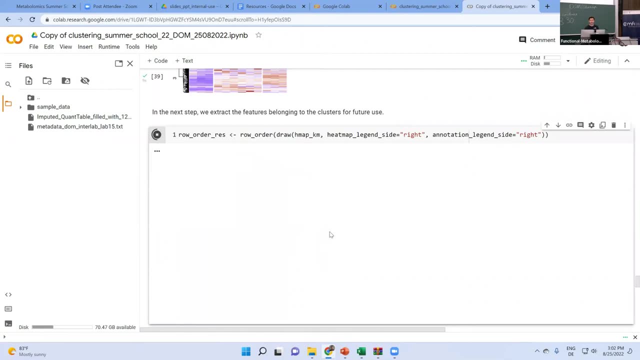 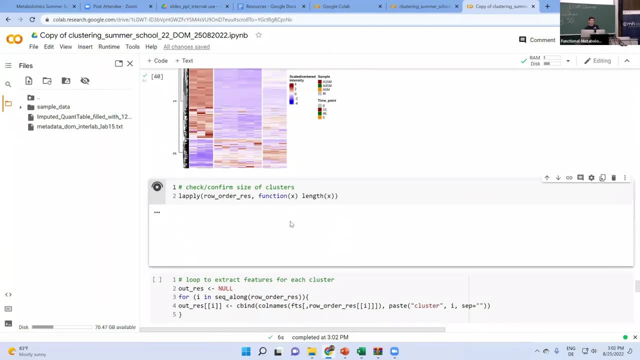 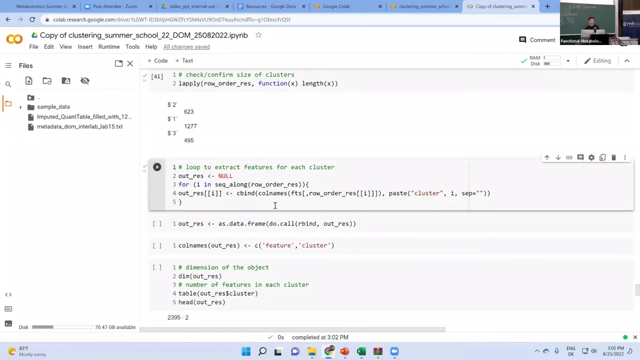 a way to extract the features that belong to a specific cluster, because I think you can use it in the future if you want to combine your results from gmps or series of any other annotation system. so I want to check how many again, how many features I have in each cluster and then I just extract them from this. 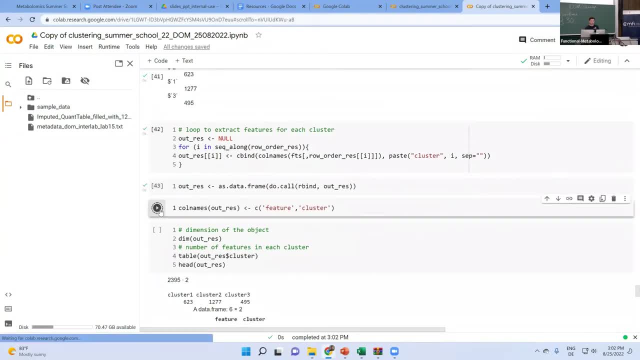 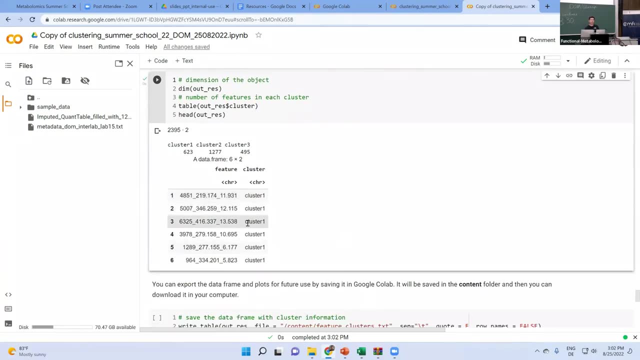 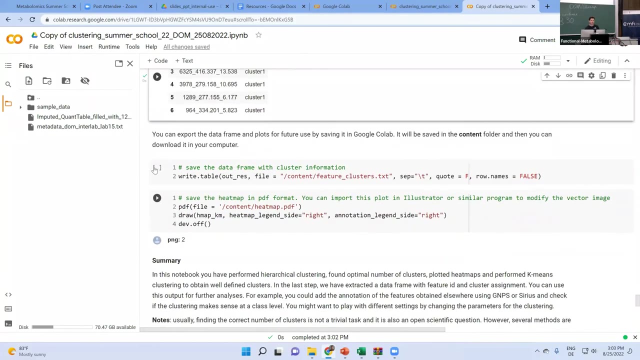 object. what you should be able to see at the end of doing this is a table with the features and the cluster assignment. it's working nice, and then you can write the file and that's it basically. you can save the PDF and go maybe in illustrator and. 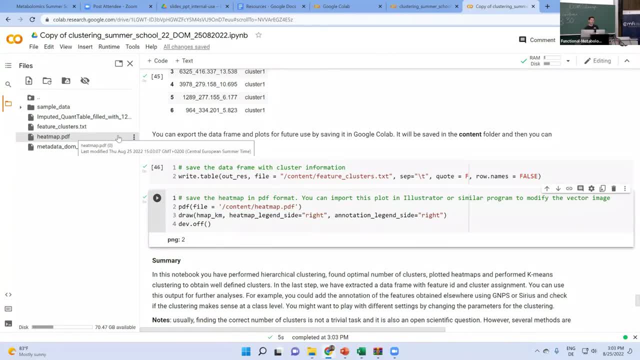 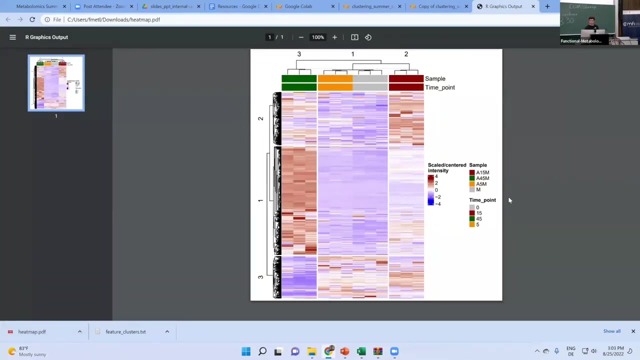 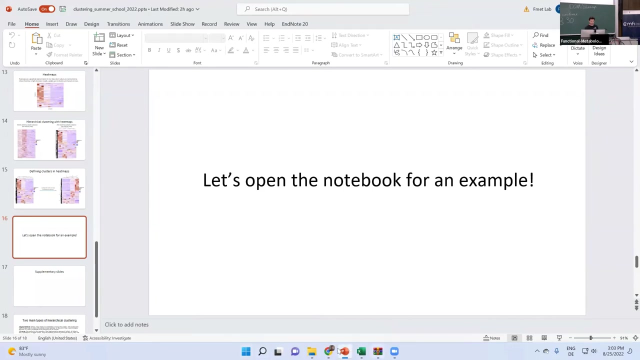 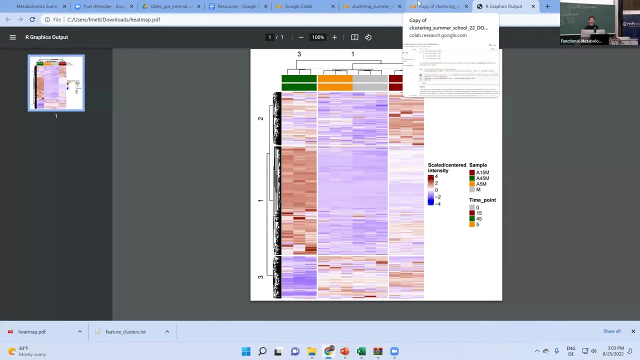 modified it or whatever you want. it is important that you download these files because they will disappear once you close, so remember to download the feature clusters and the ITMA. so it's working. you can open it and see how it the result. it's not, Thanks. 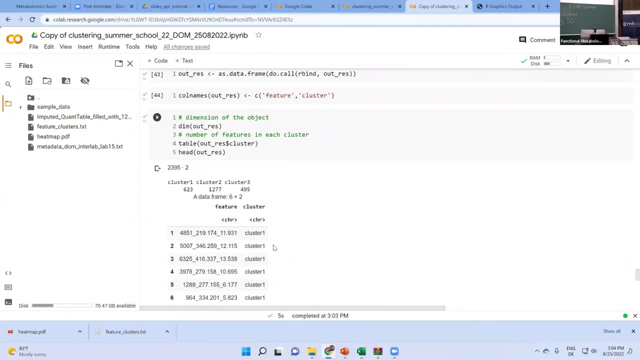 Someone else has problems? Yeah, So if you want to publish your paper while you are using this, would you then scale? Or, like the question about the details, would you then scale Another book or I will share, I will share everything. 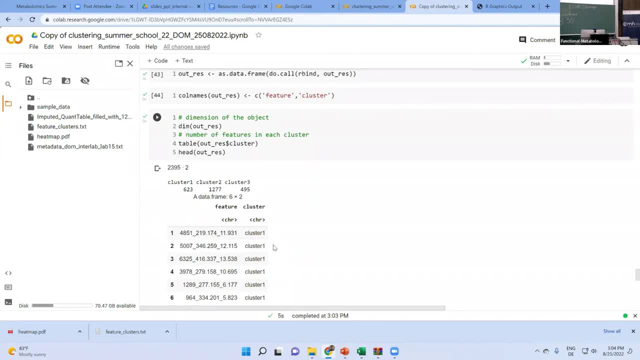 So from the notebook to the PDF files, if you want to include them in the paper. Otherwise, just the notebook that you generated will remember all the plots and all the other commands. I usually will share it as a notebook or as an HTML file for PDF. 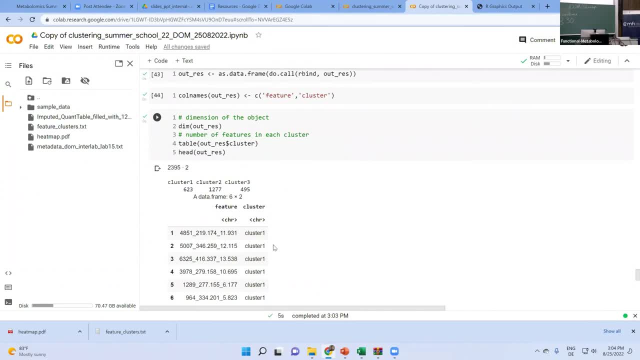 So then people can just open it without the need of knowing Google, Colab or Anaconda or anything else. You can download it as an HTML file. Nowadays, journals require to release the code in most of the journals, So you really need to think about how reproducible are your results, I guess. 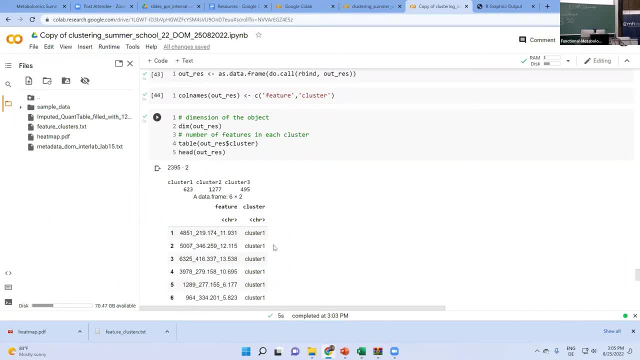 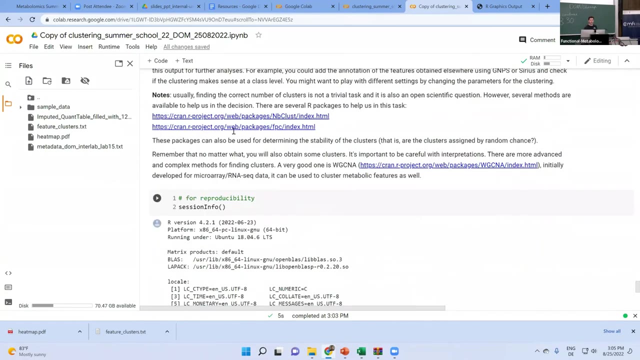 And I will share also my content: environment, if I was working with my computer so that people can install my environment as well. So it's exactly the same. Actually, at the end of this notebook, you can see here, You can see here that I'm saying: I want to see all the versions and all the stuff that I'm running.